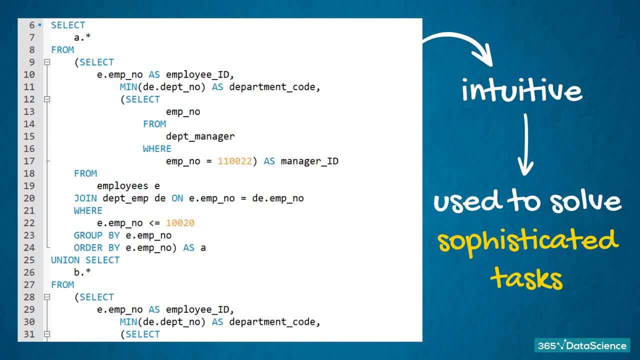 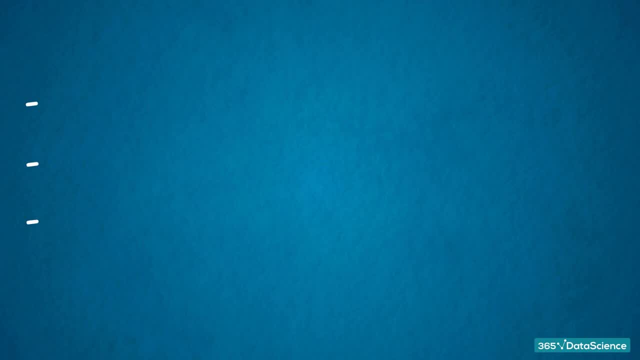 want to grasp the wide scope of its application and the ease with which this language can solve sophisticated tasks. Therefore, in the first part of this course, we will focus on explaining databases, database management systems and SQL. I have organized the videos so the abstract ideas are easy to understand. No, this will 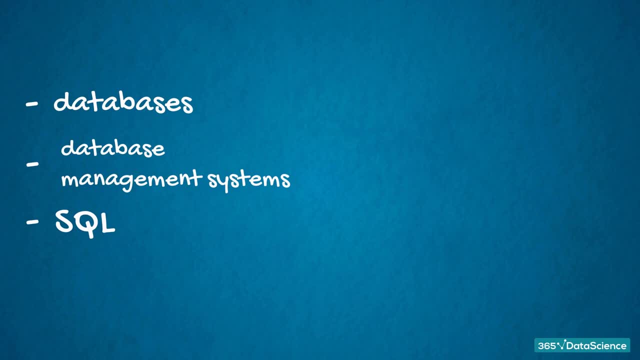 not be a set of boring theoretical SQL concepts you will never hear at your workplace. This is precisely the knowledge you need: to understand how to work with data tables, relational database management systems and their visual representation. Before we start, I would like 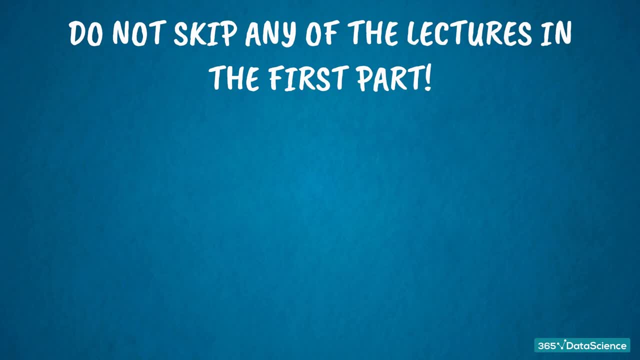 to ask a favor. Do not skip any of the lectures in the first part. I promise they will help you develop the perfect orientation and logical reasoning required for smooth, high-quality coding throughout the course. After the first part, we'll show you how to set up the software environment. you'll 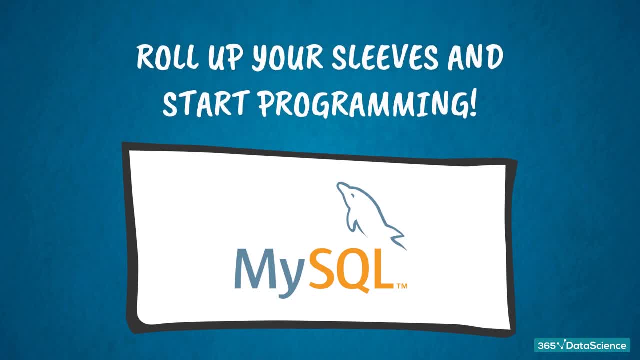 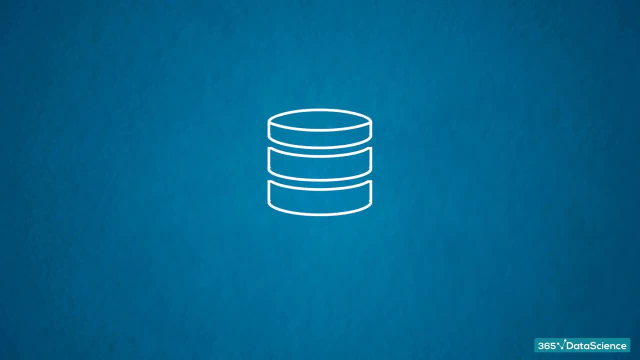 need in this course And you'll be able to roll up your sleeves and start programming. The best part is you won't just see how you can work with an existing database. We will show you how to create an entirely new database from scratch. That's great, right. 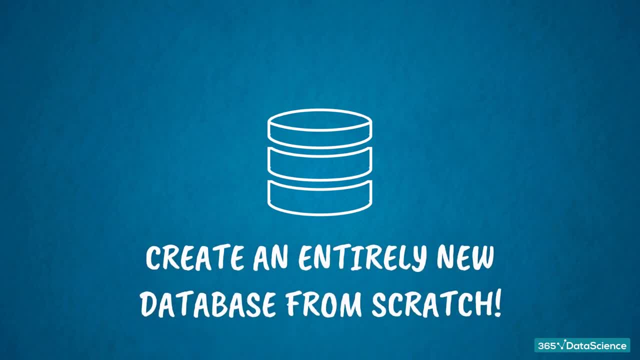 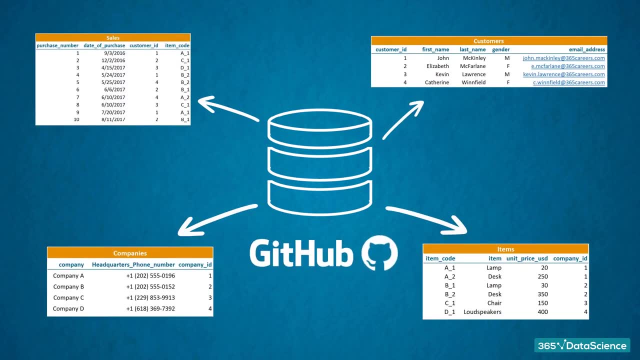 I hope you will enjoy this video. Thank you for watching. See you next time. Just wait to hear what comes after that. In this course, we will work with a real-world database from GitHub. It is large enough and will give you a good idea of how we can use SQL in real-life situations. It is not a small. 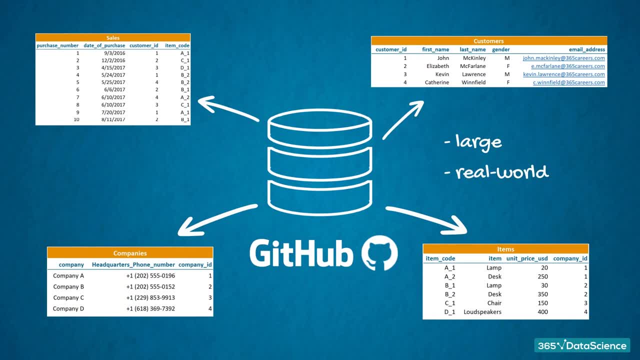 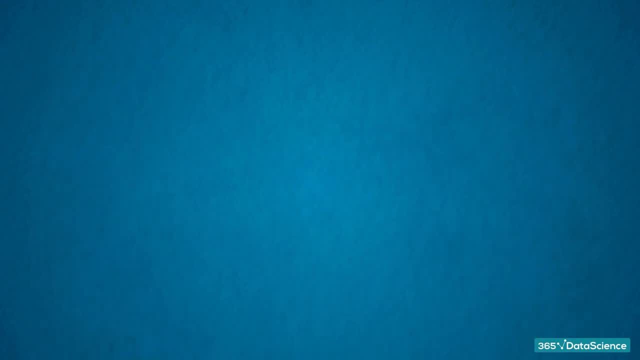 data set gathered for a beginner's course. I am sure you will appreciate this aspect of the course. We believe this is the right way to learn SQL. Then, after you have learned how to set up a database on your own, you will plunge into. 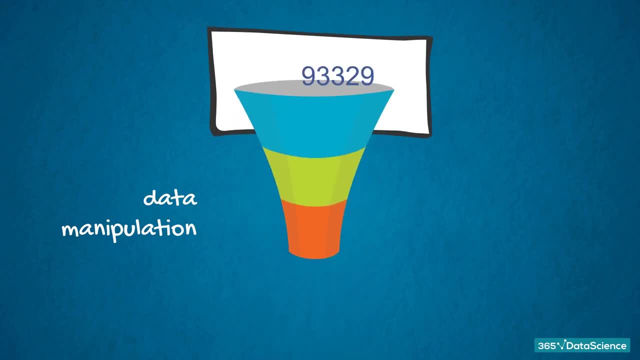 the wonderful world of data manipulation. This is the section where you will learn how powerful SQL can be when used for the extraction of information and insights from a database. You'll go through the classical SQL statements, column and table constraints functions. Then we will cover more sophisticated topics such as joins, sub-queries, self-joins and 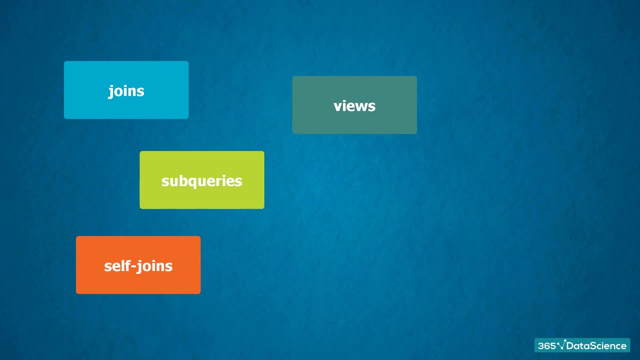 views. Finally, we'll be ready to learn how to work with some tools professionals love to use: stored procedures and functions. We will conclude the course by learning about a few challenging advanced SQL techniques, such as triggers and indexes. Besides the fundamentals, this course will teach you a solid set of useful topics tips. 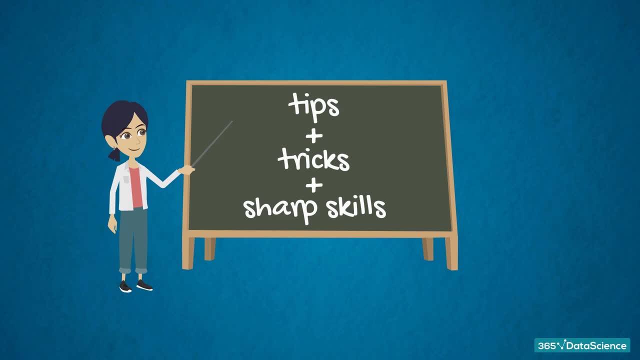 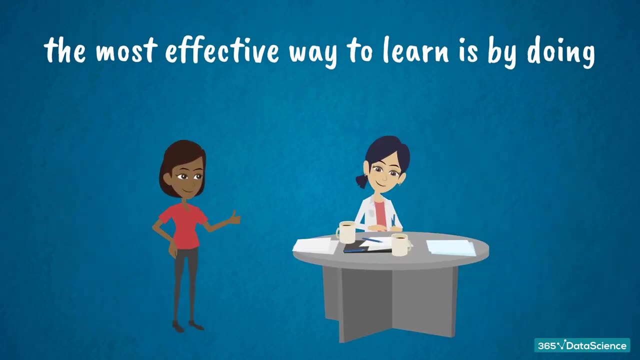 tricks and sharp skills that will give you an edge in the market. I am a firm believer in the statement the most effective way to learn is by doing. This is valid especially for SQL, because the difficulty of the tasks you must deal 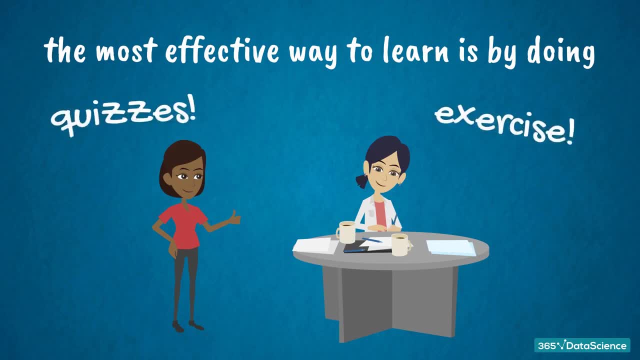 with at work require previous experience, So please do the exercises attached to the lectures. They will be in the form of quiz questions and will reinforce everything you have learned in the lessons. In addition, throughout the course and in my practice, I stick to best practices and 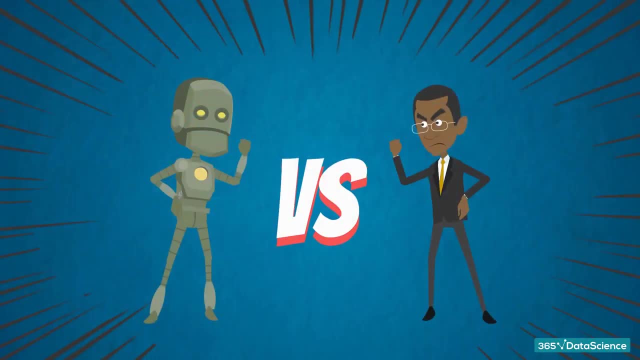 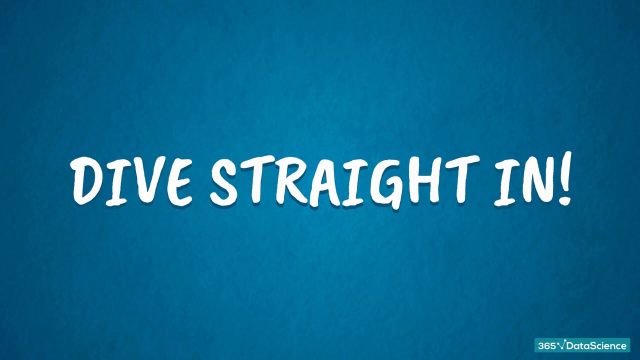 clean coding. Remember: a well-organized or good code is not the one computers can understand, it is the one humans can understand. So what are you waiting for? Dive straight in and let's begin this journey together. So why study SQL? 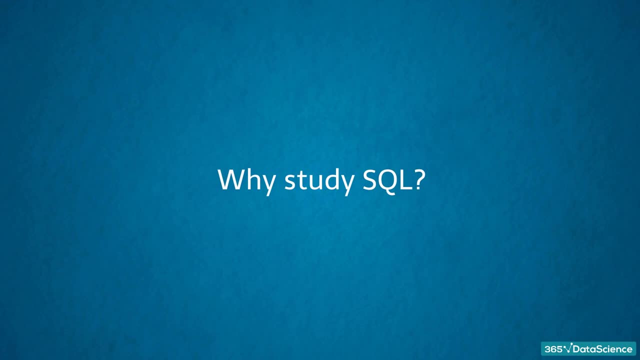 Put yourself in the shoes of an employee or a manager of a company who works with large amounts of data. For example, you could be working in business intelligence, BI, data science, database administration or back-end web development. Any of these jobs relate to storing large amounts of data. 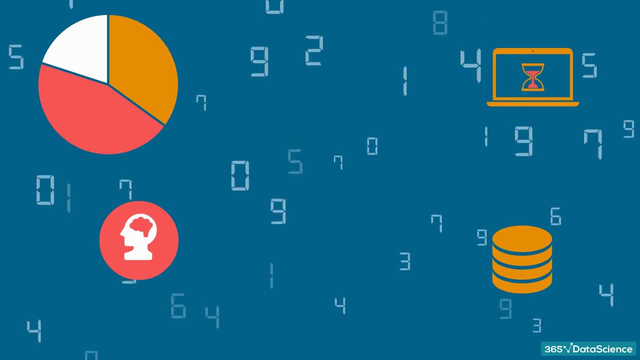 Therefore, before carrying out any analysis with the data, you will have to retrieve it. As a consequence, the focus of this course will be on storing large amounts of data. So why study SQL? The purpose of our course is namely on developing the skills required to solve business analytical. 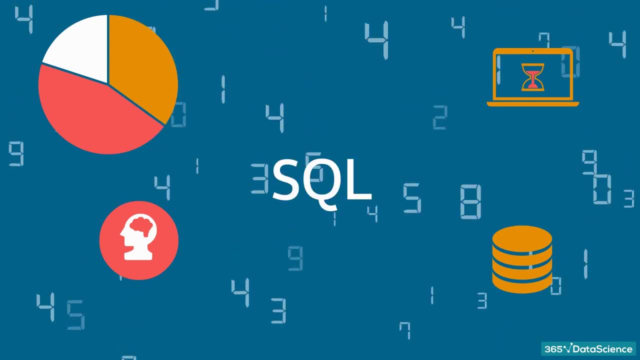 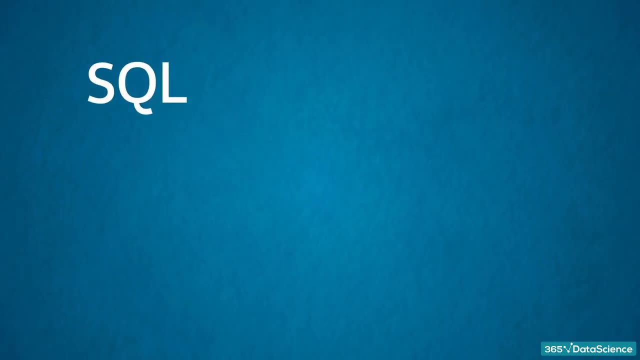 problems and applying solutions in a software that allows you to extract the desired information from the database. To achieve all this, you need SQL. SQL means Structured Query Language. It is a programming language specifically designed for working with databases. It allows you to create, manipulate and share data, especially data from relational database. 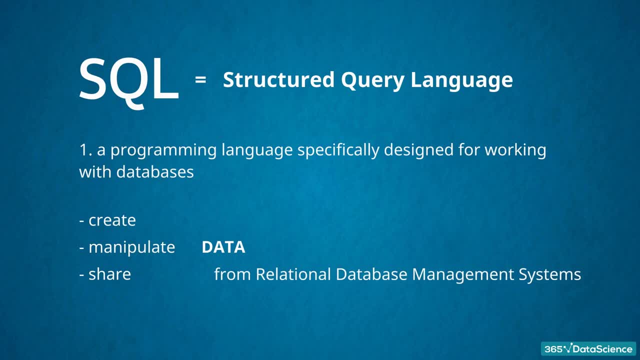 management systems. The way to tell the computer to extract information from the database is by using SQL. The way to tell the computer to extract information from the database is by using SQL. The way to tell the computer to extract information from the database is by using SQL. 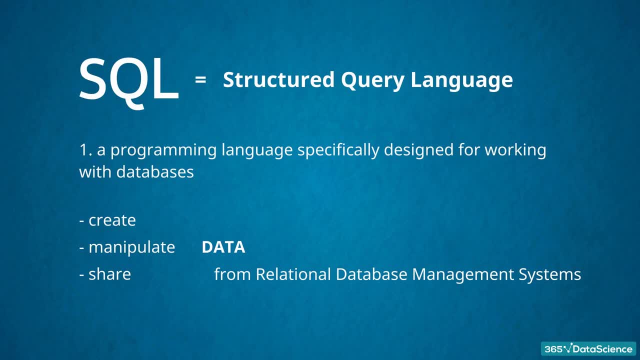 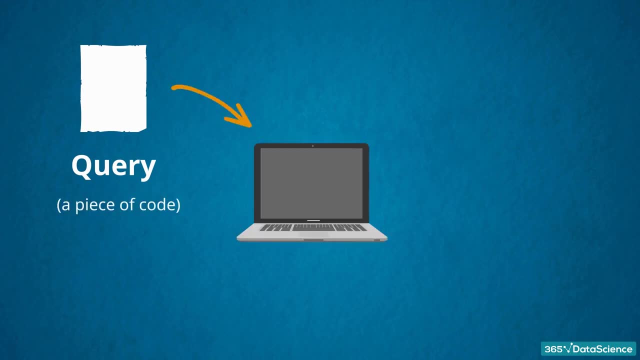 A query is a piece of code inducing the computer to execute a certain operation that will deliver the desired output. The latter process is called querying the database. Briefly, SQL is the language that allows you to write queries that the computer can execute and then provide database insights in return. 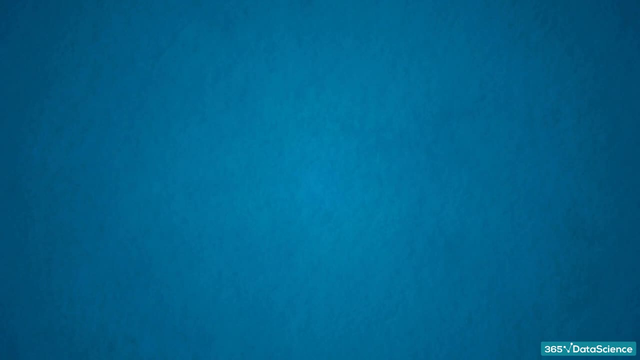 In MANCAP. SQL is a language that allows you to write and execute queries that the computer can execute and then provide database insights in return. The good thing about SQL is it is an intuitive and easy-to-learning language. to learn language- Be careful, as this does not mean using it will be a simple task. 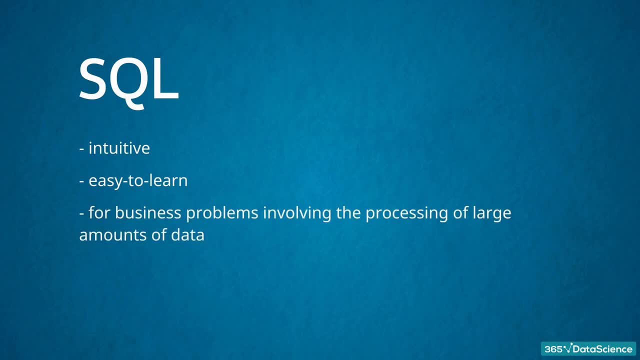 Not at all. Sometimes, the business problems you must solve will be peculiar and will involve the processing of large amounts of data. Despite being relatively simple in its structure, SQL can be powerful while computing complex tasks. This is why, in this course, we provide the raw skills you'll need to become a web programmer. 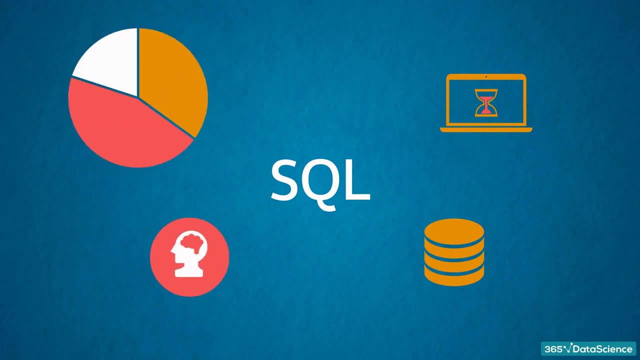 a data analyst, a data scientist or a business intelligence analyst. The idea is to combine video lessons and advanced exercises that will show you SQL's cool and fun to work with And if, for some strange reason, you are still wondering whether SQL is a programming language, 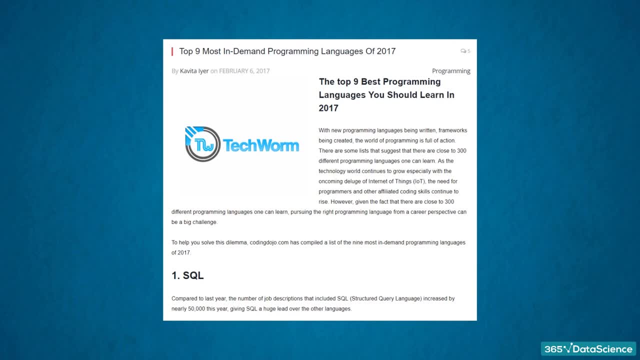 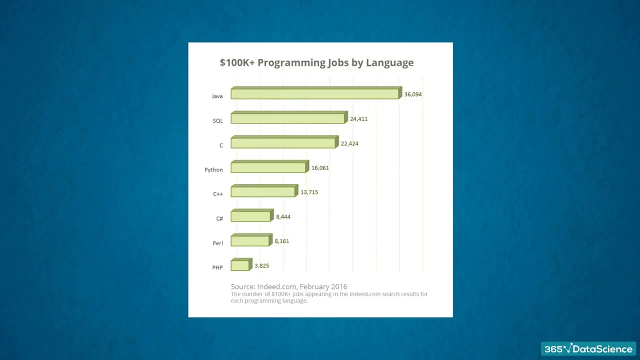 worth having in your skill set. let me show you the following statistics. A TechWorm study shows SQL is the most demanded programming language for 2017.. In general, not in a specific sector. Indeedcom shared the same information for 2016.. 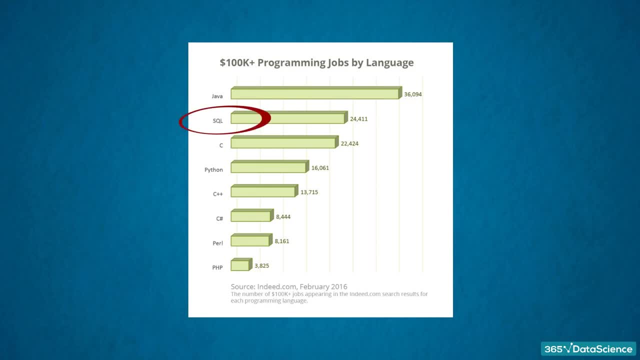 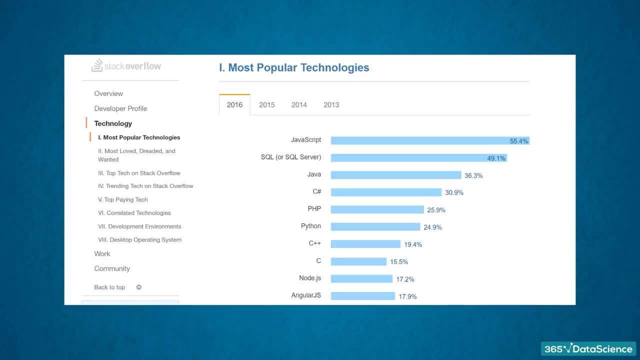 Indeedcom also ranks SQL high when related to lucrative job positions. It is true, Sometimes these kinds of studies are indeed biased, So let's change the question and refer to a study conducted by Stack Overflow, where they asked over 56,000 developers in 173 countries which are the most used technologies. 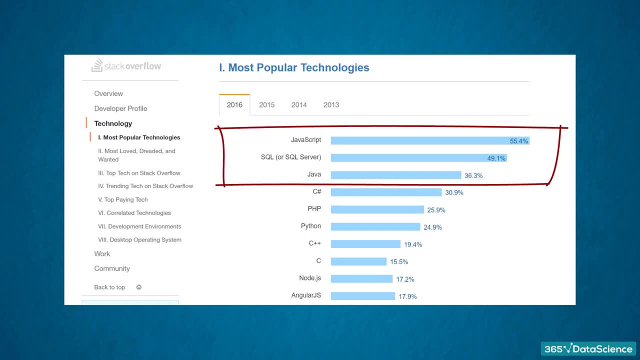 The top three are…: 1. JavaScript – 55.4%. 2. SQL – 49.1%. 3. Java – 36.3%. Therefore, SQL is a highly demanded skill in the job market, no matter how you look. 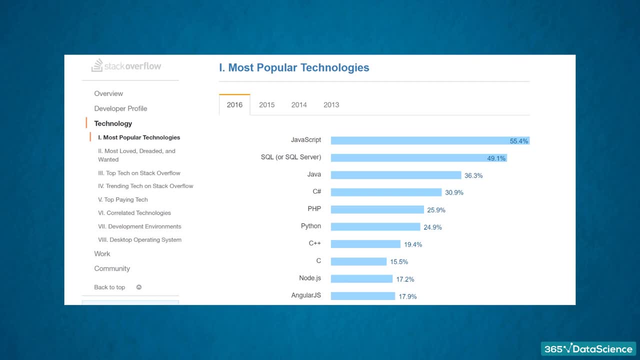 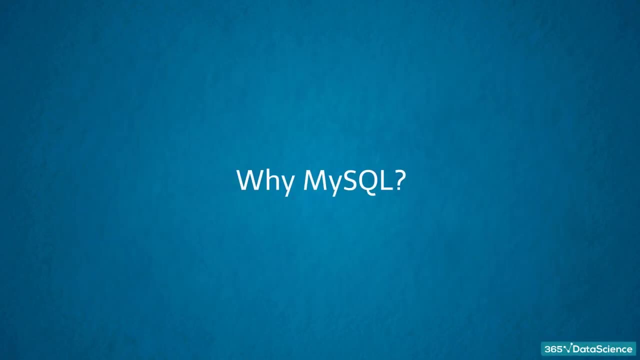 at it. Stay tuned for the next video to understand what it is and why it is the most suitable software environment for this course. Ok, so At this point you might be telling yourself… Great, Let's start with the SQL. If you want to learn more about SQL, you need to learn how to use the software. you're 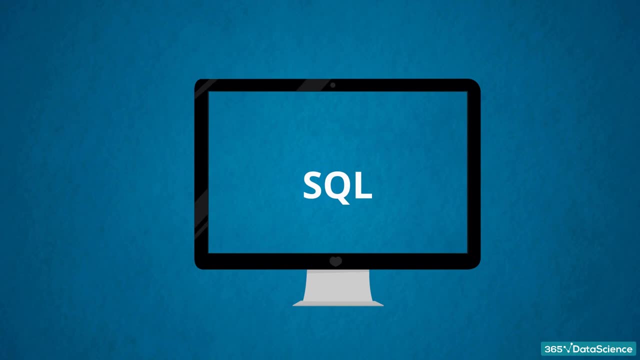 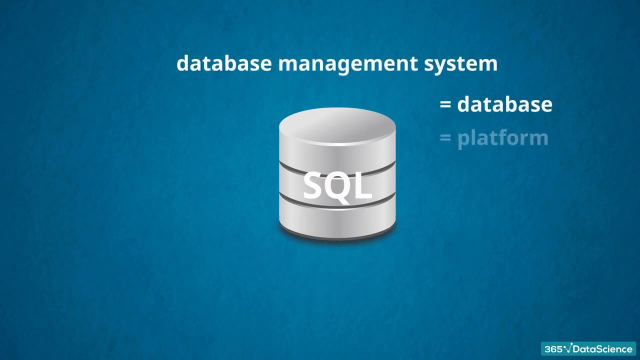 using. You can use the software you're using to start your course. Unfortunately, it is not so simple. Why? To implement SQL commands, you will need a database management system, often called a database or a platform. The problem is there are a few popular databases out there which are all based on SQL. 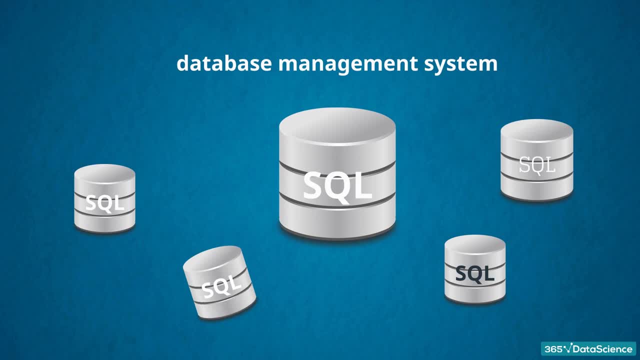 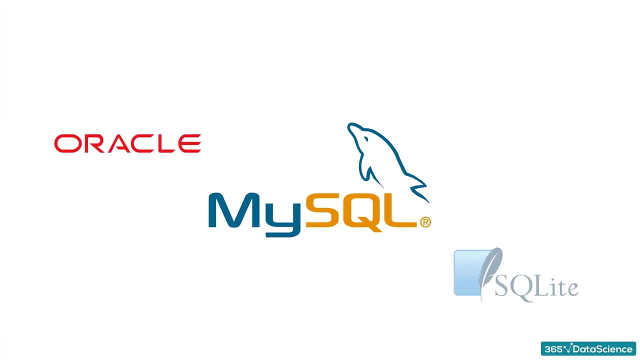 They support various forms of the original language and there are only slight differences between different versions. As a developer, you want to learn how to use the one that is the most suitable for your situation. We will base our course entirely on MySQL, But you should know there are other platforms like Oracle, SQLite, Microsoft SQL Server. 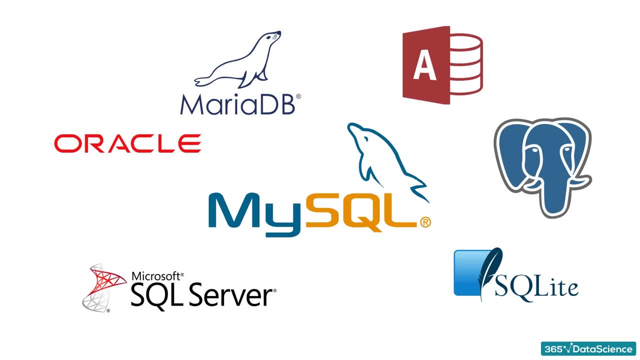 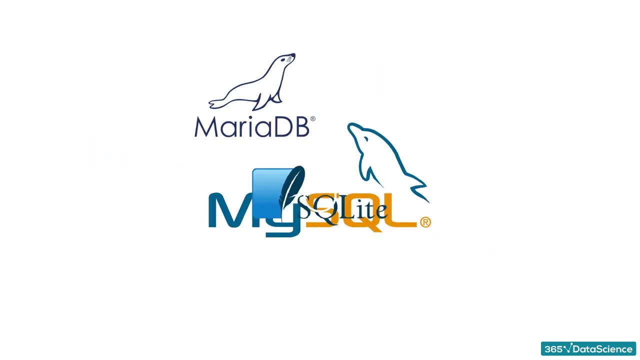 PostgreSQL, MariaDB, Microsoft Access and so on. The minor differences between the versions of the SQL language mean that transferring from one database to the other, which usually happens if you are changing jobs, would not be an obstacle for you. If you are a user of another platform, you can still take this course and easily apply. 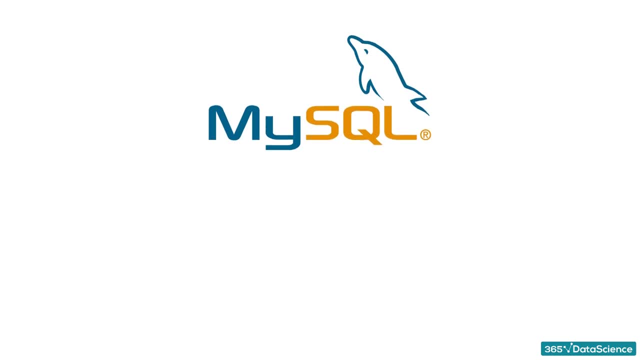 the tools we teach. So why do we choose MySQL? Because it is reliable, mature and open source. The latter means it is free. It is used by many institutions and companies, including Facebook, YouTube, Dropbox, Twitter, Pinterest, Bookingcom and LinkedIn. 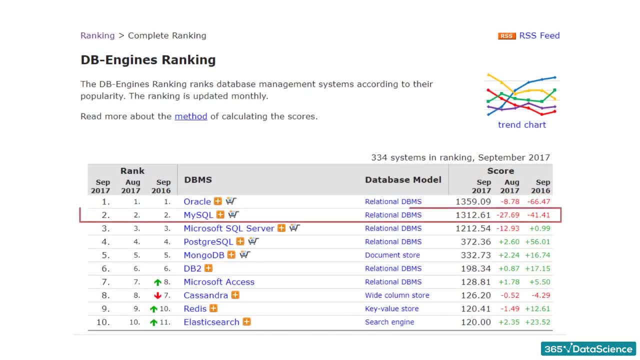 Considering the well-renowned DB Engines ranking, MySQL comes as the first open-source relational database management system. Yes, MySQL is on top, with only a slight advantage. but don't forget, it is a paid software. Therefore, aiming at providing you with the best experience possible, we chose MySQL. 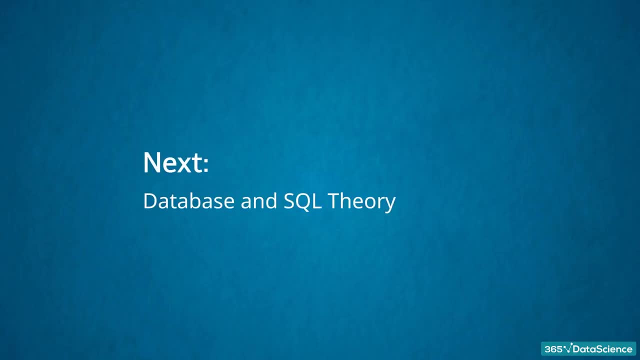 Now let's dig into some database and SQL theory. This will provide the set of tools you'll need when we deal with various SQL tasks in the lessons to come. All right, great. One thing you'll notice when studying programming languages is that the concepts that we are 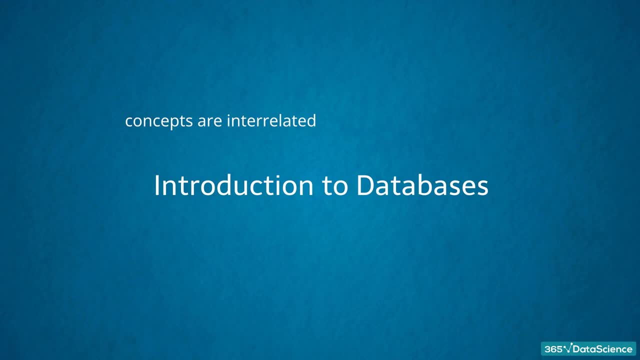 talking about are interrelated. This means focusing on a single topic can hardly deliver the content that must be explained in its entirety To this story. SQL makes no exception. Despite that, we must start from somewhere right. My working experience tells me you will be much faster in learning and writing efficient. 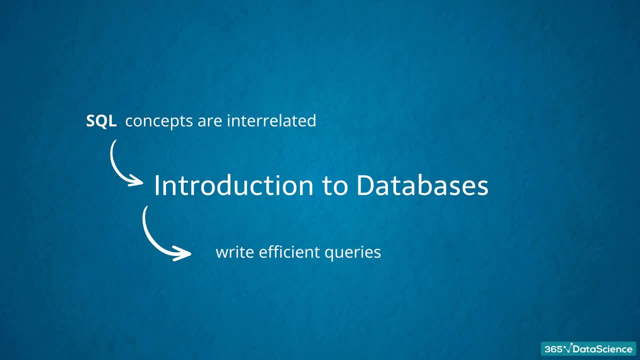 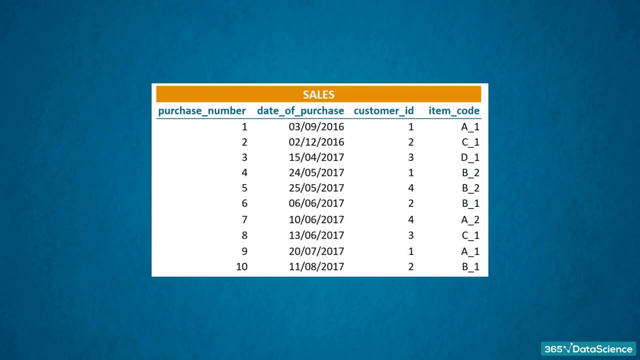 queries. if you go through a brief introduction to databases, It is the best thing to begin with. so here's what I would like to share with you. The table you see here contains data. The table contains data about the customer sales of a furniture store. 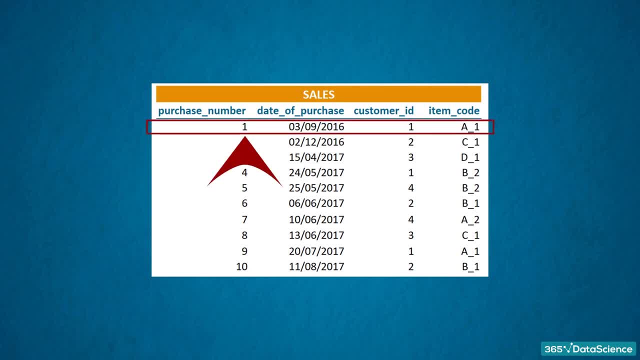 And this is how we should read this information: Purchase number 1 was registered on the 3rd of September 2016.. Then customer number 1 bought the item with code A1.. Each of the four elements has a specific meaning. 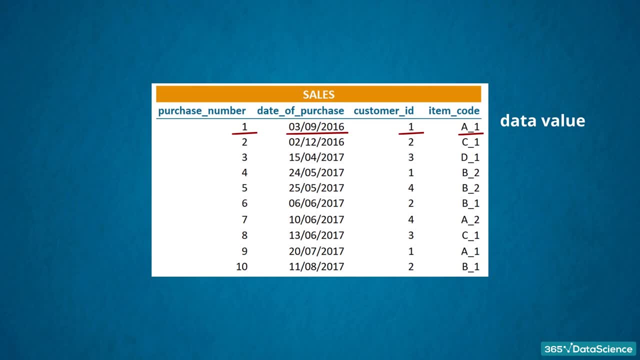 We will call each one a data value. All four data values make up one record. A record is each entry that exists in a table. It corresponds to a row of the table. Therefore, these four data values form one record and these data values regarding purchase. 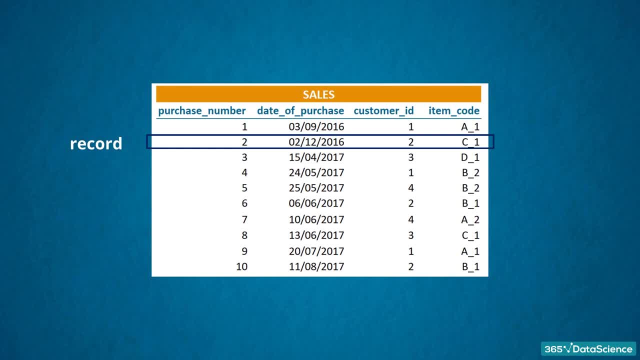 number 2 form another record. You could use the terms row and record interchangeably. Besides the rows, you can see the data is separated into four columns or fields. A field is a column in a table containing specific information about every record in the table. 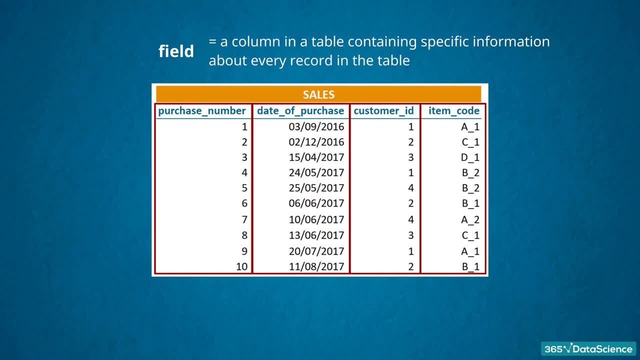 This means all the records in a table, regardless if they are 10,, 10,000, or 10 million, will have a certain purchase number, date of purchase, customer ID and item information. When the data you have is organized in rows and columns, this means you are dealing with. 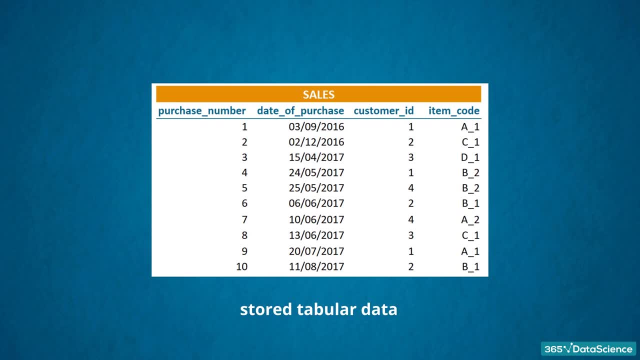 stored tabular data. That is important to mention because you will often see in the literature that database management relates to data stored in tabular form. Great, Here comes the more interesting part In this table: we know nothing about a customer besides her ID. 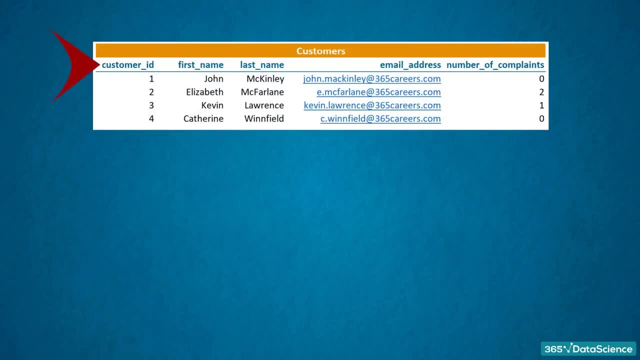 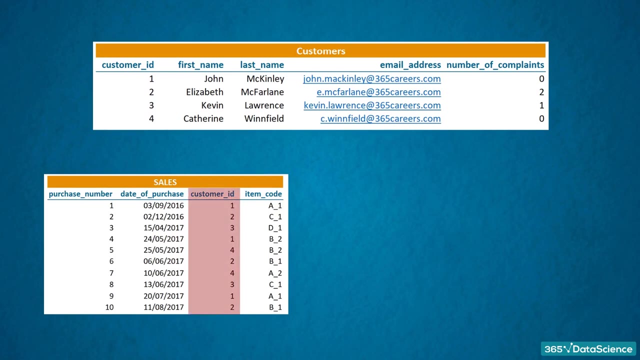 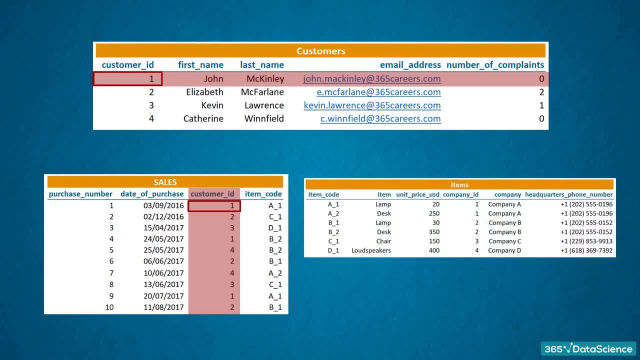 the pure example we have for a customer. After all, information about customers is stored in an list of item files. It contains the item code, product description, its unit price ID and name of the company that has delivered it and the company's headquarters phone number. 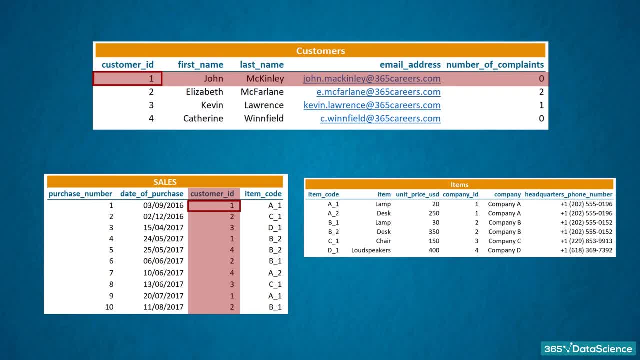 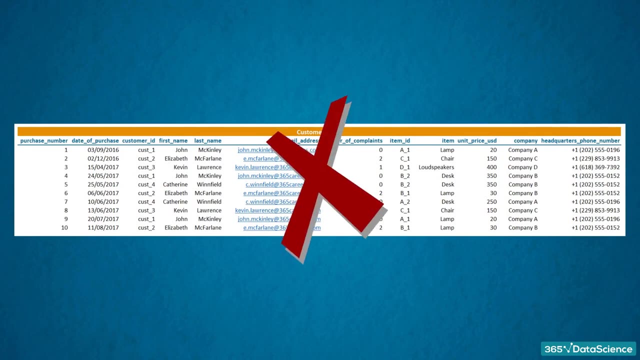 Here, the connection between the sales table and the items table is not the customer ID but the item code. Well, we could stuff this information into one table and it would look like this: Ouch, It is huge. I would not want to imagine what the table would look like if we had registered over 10 rows. 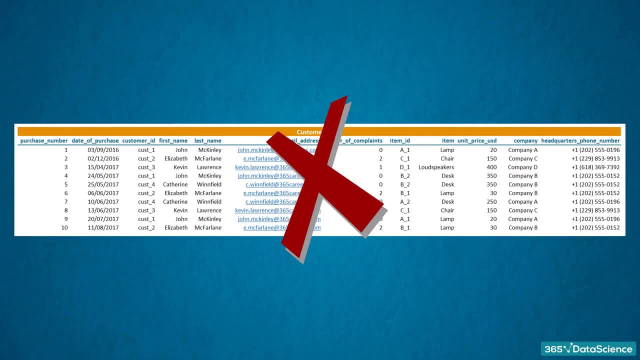 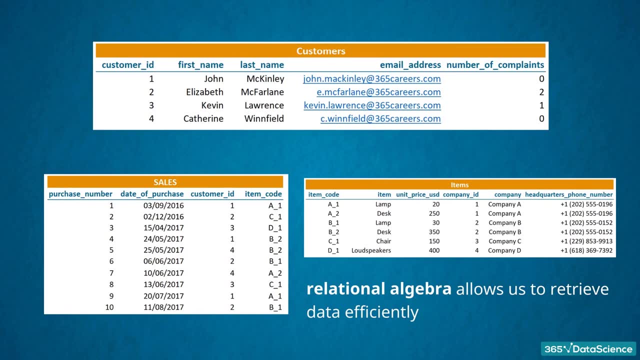 My point is: there are too many columns and it is hard to understand what type of information is contained in the larger table. Relational algebra allows us to use mathematical logic and create a relation between a few tables in a way that allows us to retrieve data efficiently. 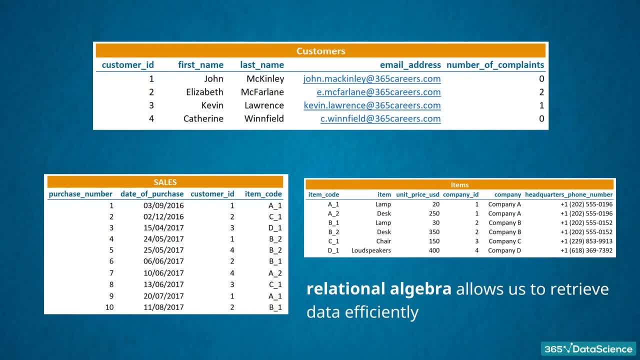 Namely these three tables: sales, customers and items are related through the customer ID or the item code columns and form the table. A few tables form a relational database and, importantly, each one bears a specific meaning and contains data characterizing it. 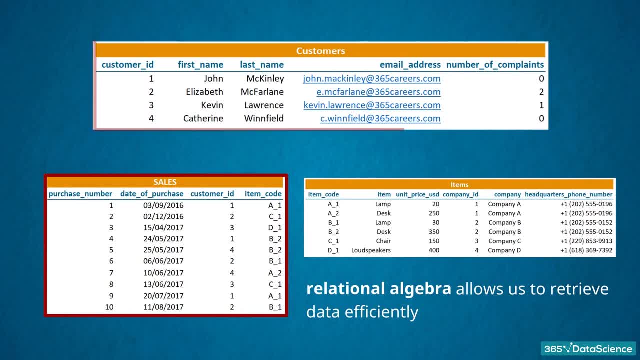 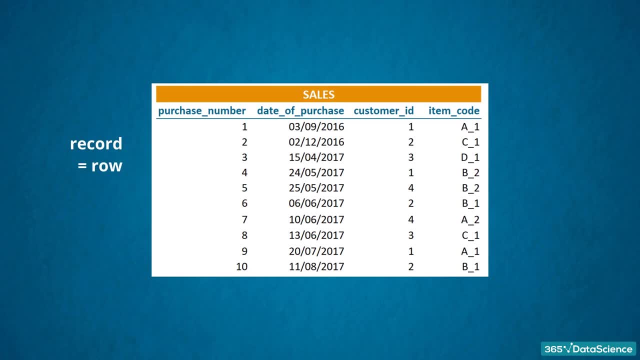 One of the tables contains information about sales, the other about customers and the third about the items. To recap, remember the data values in a row form a record in a table, and each column represents a field that carries specific information about every record. 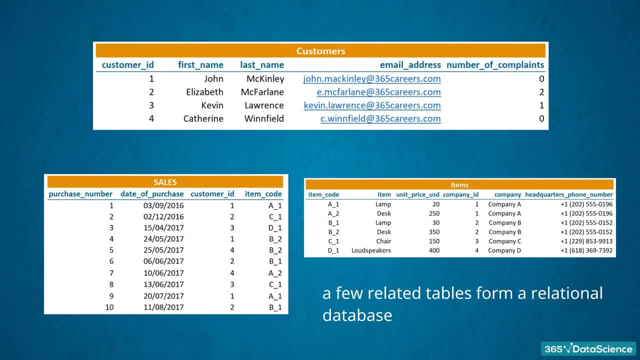 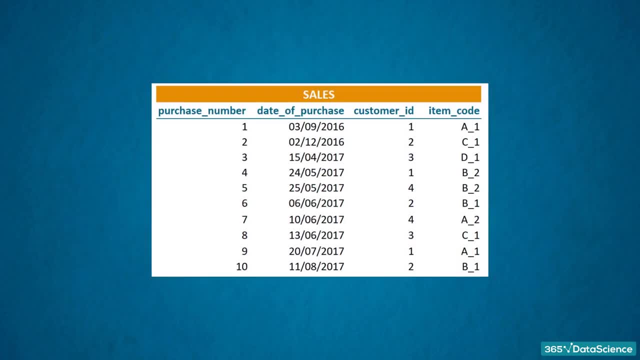 A few related tables form a relational database And for those of you who are interested in slightly more technical definitions, remember the smallest unit that can contain a meaningful set of data is called an entity. Therefore, the rows represent the horizontal entity in the table, the columns its vertical entity. 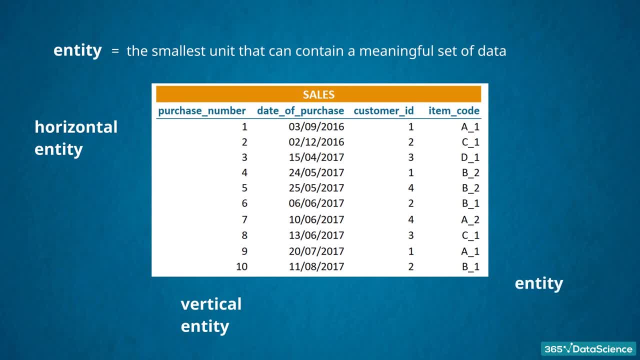 The table is a bigger data entity. on its own, It can also be referred to as a database object. A single row of a table being a single occurrence of that entity can be also called an entity instance. Ok, great, We will gradually build the theoretical preparation you need before you begin coding. 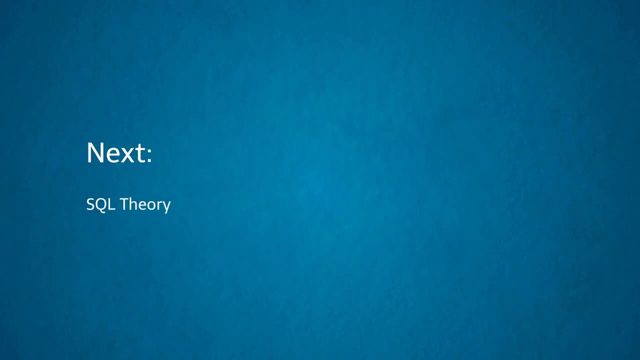 Stay tuned for the next lecture, where you'll see Aались's role when working with relational databases. Now that you know what a database is and have an idea about how it works, it is much easier to understand how SQL fits in the whole picture. 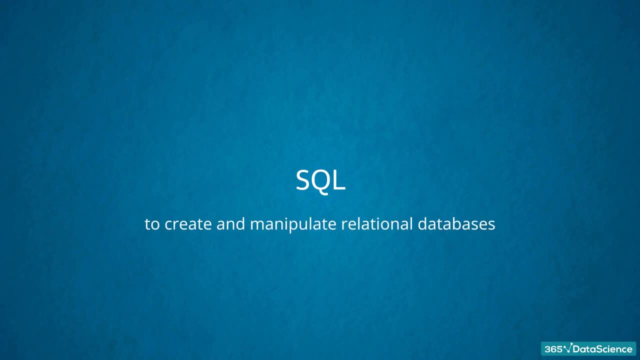 SQL is the programming language you need to execute commands that let you create and manipulate relational databases. The Friedman and Rabi book one is the only one you'll read. There are a million other options combined to solve this question. Your order will be also flat. Crit UNIVERSAL FRIED may cost tripled Hmph delayed, Never mindgesetz is driving you out. There's all there to do, then cdc. 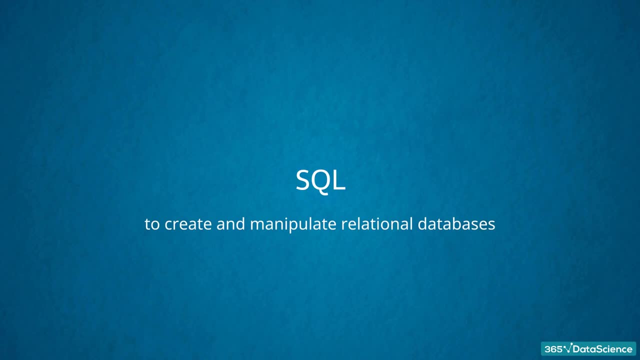 database. We will not delve into strict and detailed technical definitions to explain how it works. What you need to know is there are a few types of programming out there – procedural, imperative, object-oriented, declarative and functional. Although with some procedural elements, SQL is mainly regarded as a declarative programming. 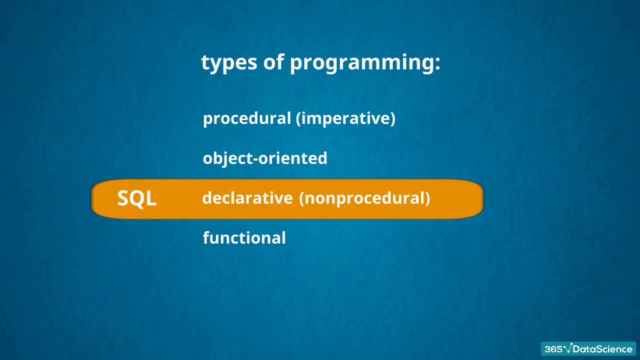 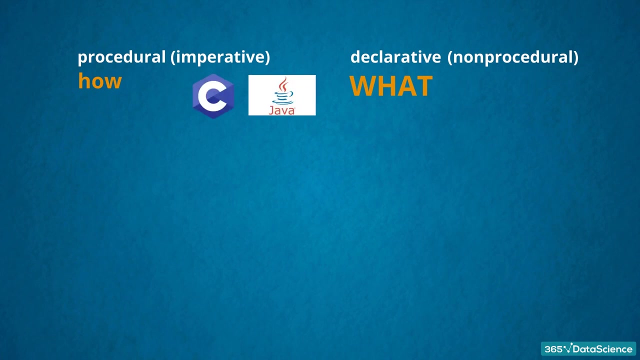 language. it is non-procedural. This means while coding, you will not be interested in how you want the job done. The focus is on what result you want to obtain. An abstract example would best clarify what we mean here. When using a procedural language such as C or Java, you must explicitly divide the 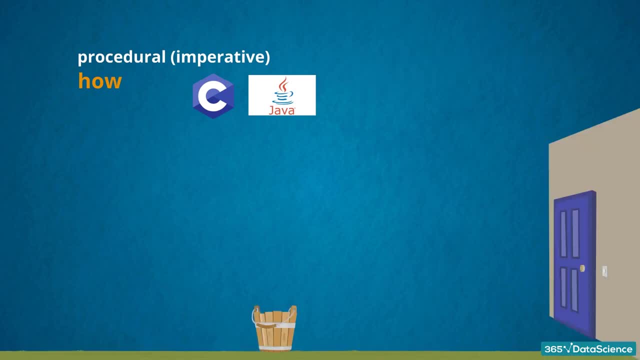 solution of a certain problem into several steps, For instance: 1. Please open the door. 2. Go outside. 3. Take the bucket I forgot there. 4. Bring it back to me. In a declarative language, this would sound like: 1.. 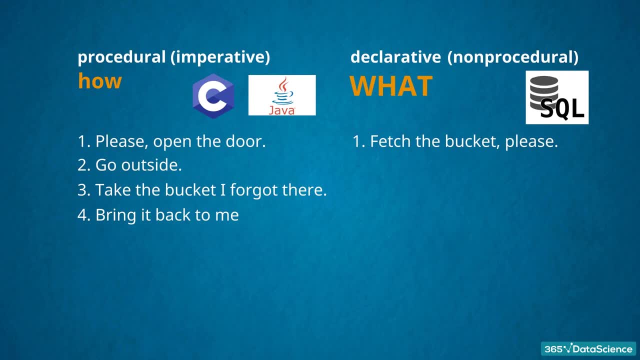 Fetch the bucket please, and you wouldn't have to go through the process step by step. The algorithms are built-in and there is an optimizer which will separate your task into smaller steps and do the magic to bring the desired output. Why is this important? 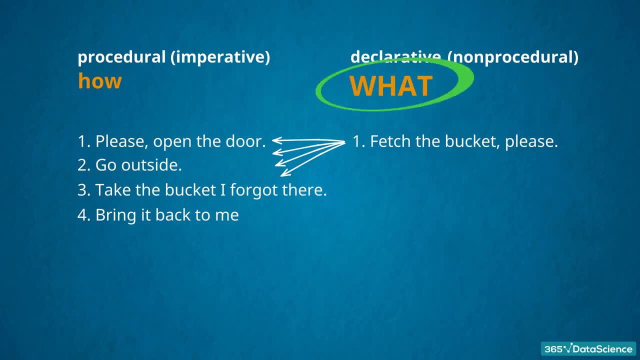 When using SQL, you should concentrate on what you want to retrieve from your databases. Unless you are an advanced user, don't bother with the algorithms explaining how your data can be obtained. Acknowledging SQL is principally a declarative language. now we can go through the main components. 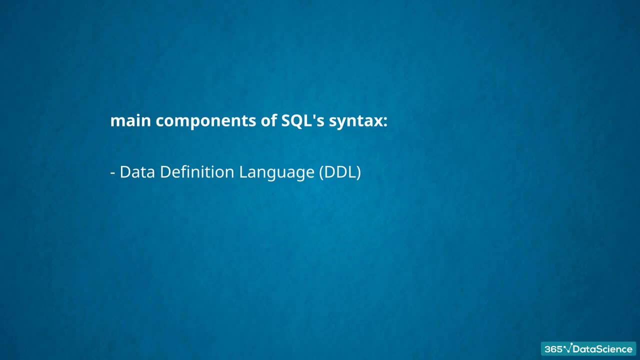 of its syntax. It comprises a data definition language known as DDL, a data manipulation language, abbreviated DML, a data control language- DCL- and a transaction control language- TCL. These will be the topics of our next few videos. 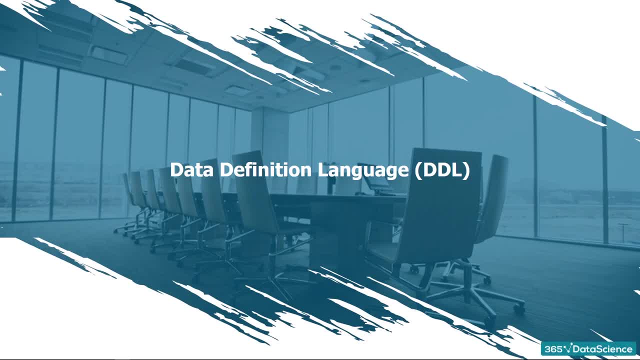 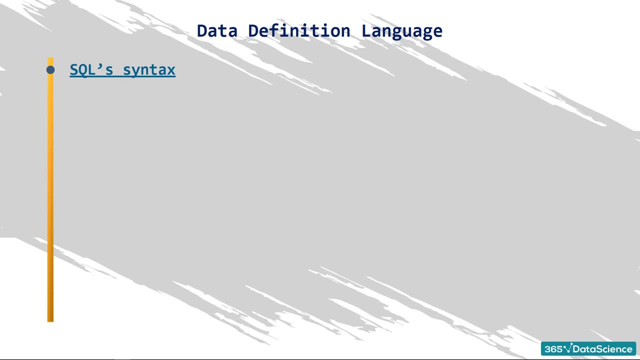 Alright, good, Let's get started. Let's go over the components of SQL's syntax. It comprises several types of statements that allow you to perform various commands and operations. The data definition language, DDL, is one type. It is called a language, but you can think of it as a syntax, a set of statements that 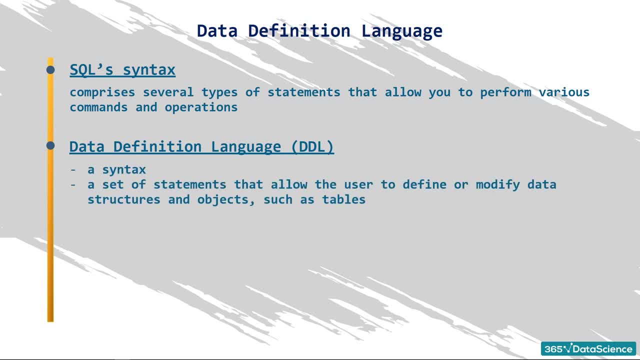 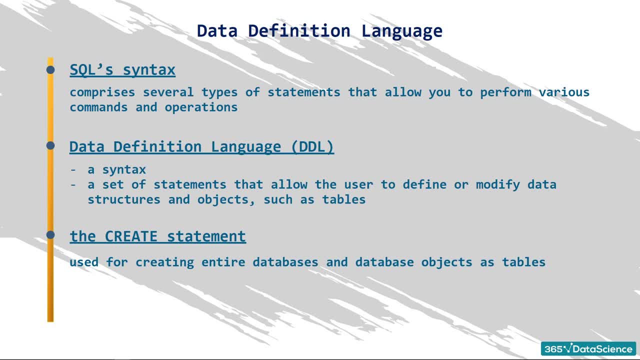 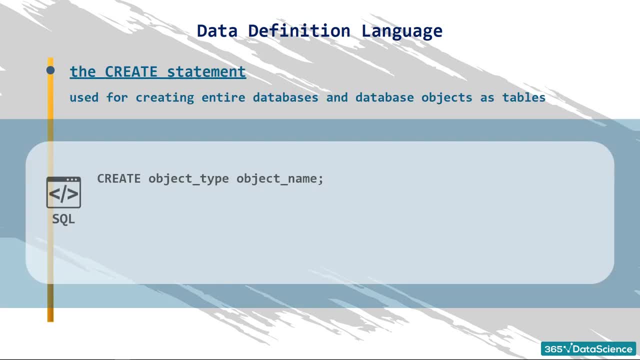 For example, if we want to create a table, we must abide by the following syntax: CREATE TABLE. OBJECT: NAME, COLUMNAME AND DATA. TYPE IN PARENTHESES AND SEMICOLUMNAM: As expected, the CREATE statement creates an object with a certain name. 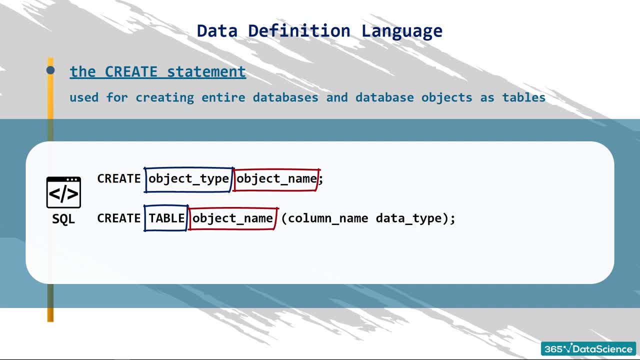 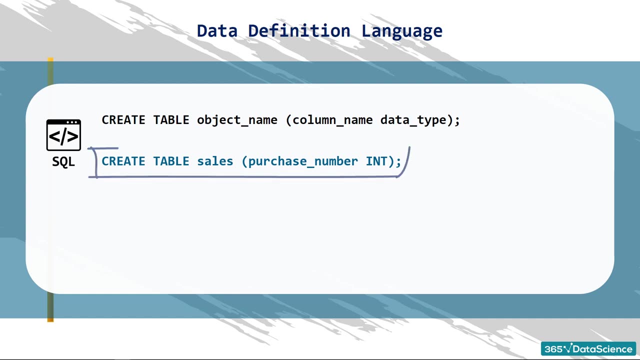 In this case, we are creating a table. Given we have to assign columns to the table. after specifying the table name, within parentheses we MUST indicate the names of the columns and the type of data contained in each column. Look at this example. With this line of code, you can create a table with: 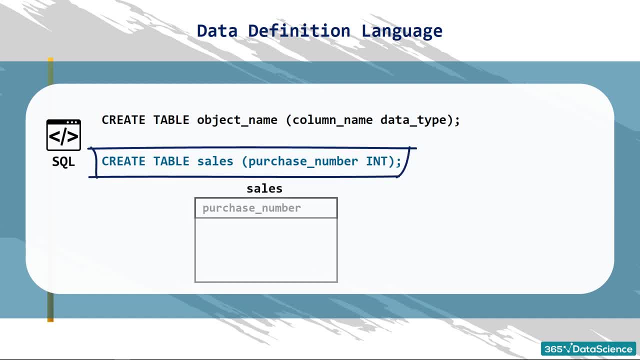 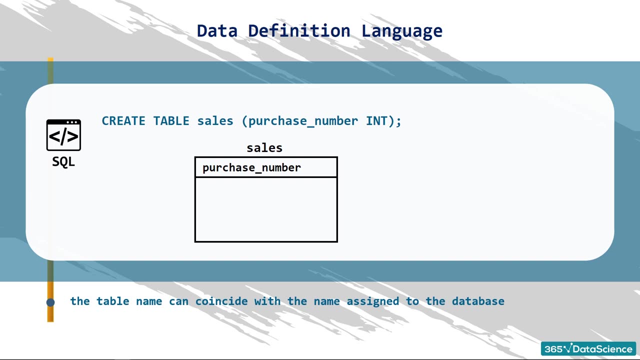 the name cells containing one column called purchase number. that will store only integer values. Easy right. Don't worry if the table name coincides with the name we've assigned to the database. This is a common practice. On one hand, the syntax will make it clearer when you refer to the database and to the table. 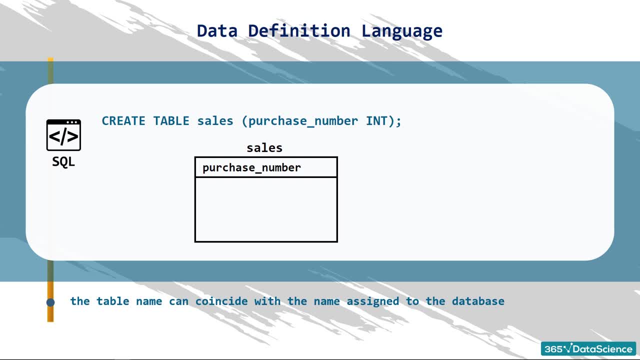 On the other hand, it is logical. It makes sense for a database to bear the same name as its main table. Okay, great. Observe how simple the syntax of the create statement is. You will have to write it at the beginning of the line. 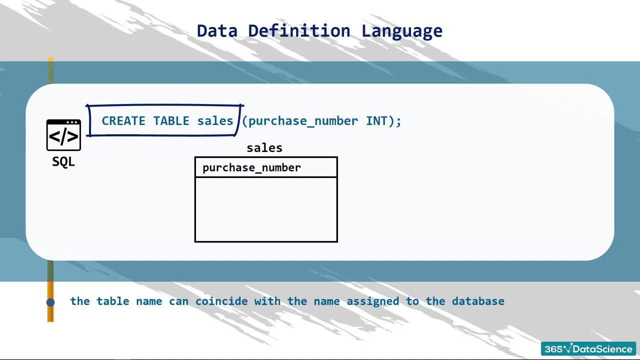 and then directly point out the type and name of the object. Awesome, And why did we start with an example where we created a table and not some other object? Because it helps us understand better how the alter statement works, which is the operation of the table. 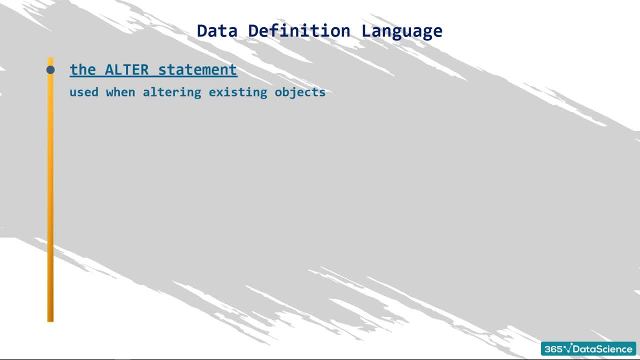 For example, we can use alter to modify a table by adding, removing or renaming one of the columns in the table. To add a column called date of purchase, you should begin with the same structure as the one used for the create statement. After alter, you will be able to designate the object type and its name. After that you are supposed to write down the precise modification. This means a new column containing the date of the purchase will be added to our table. 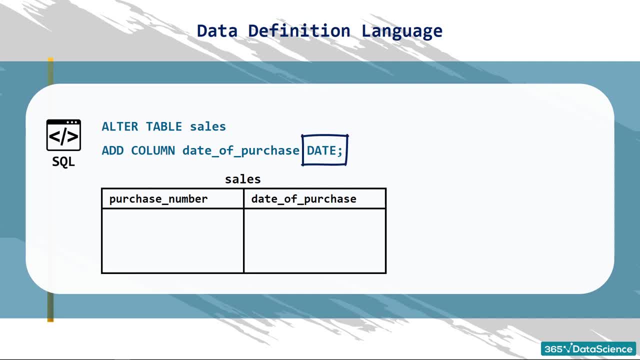 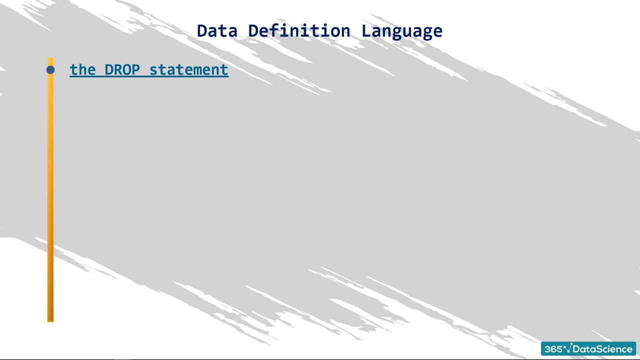 In addition, the values in this column will be of the date type: Intuitive right. What if you want to delete a database object? In that case, you can use the drop statement to do that. For instance, we can delete the entire customers table with. 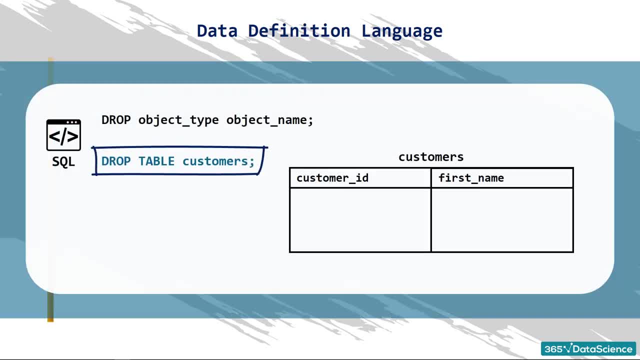 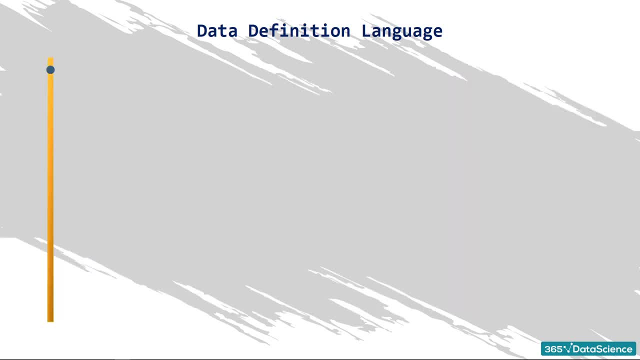 a single line of code. Drop table customers. As you can see, the DDL statement was accompanied by the object type and its name. Another valuable tool when using the data definition language is rename. This piece of syntax allows you to rename an object like a database table. 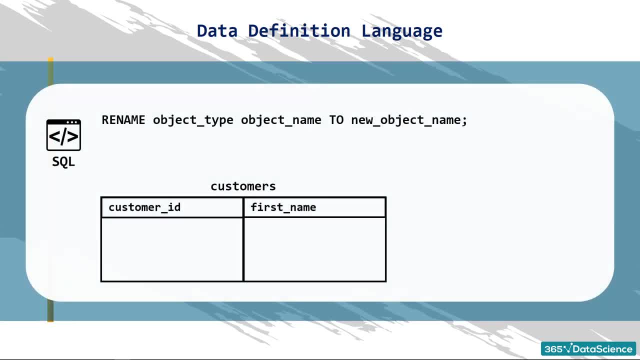 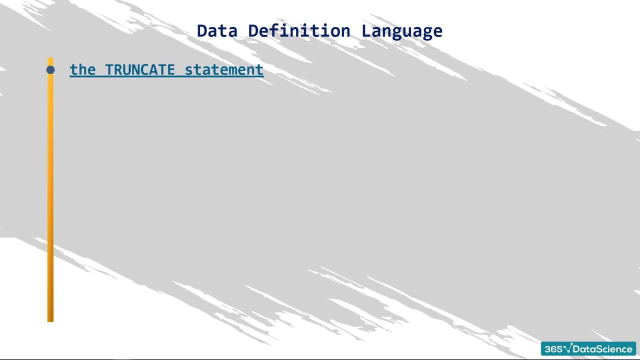 If we hadn't dropped the customers table, rename table customers to customer data would have changed the name of the table to customer data. Okay, finally, instead of deleting an entire table through drop, we can also remove its data and continue to have the table as an object in the database In. 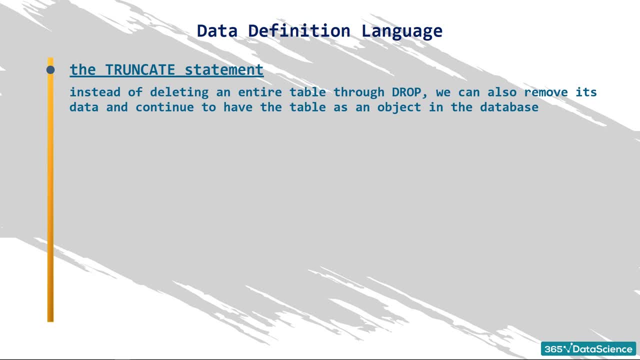 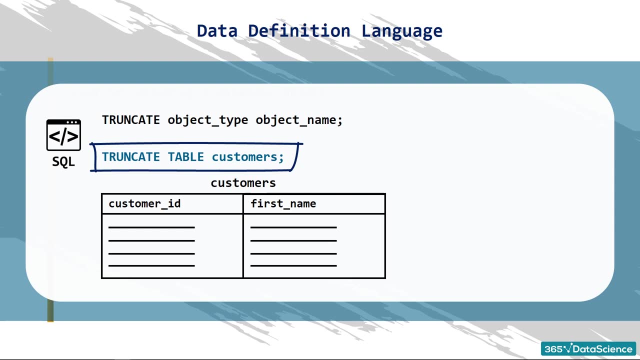 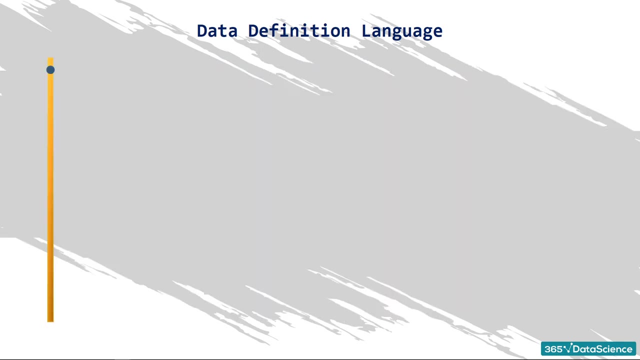 such a situation. truncate is the DDL statement that would allow us to do that. After executing this clause, all the records from the customers table will be deleted, But, although empty, the table will continue to exist. As a quick recap of this lesson, remember the data definition. language constitutes the part. 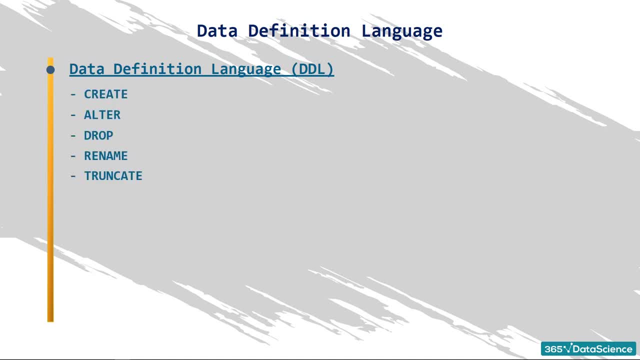 of the SQL syntax that allows you to create, alter, drop, rename and truncate databases in their elements. Once you have created a database with its elements and have loaded it with information, you are ready to step up to the next level and manipulate the data definition. 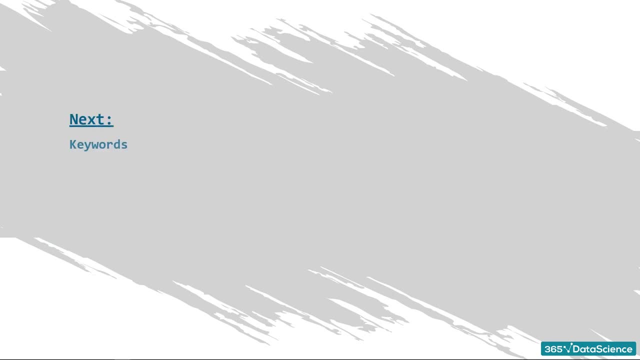 Let's stop for a quick side note. Add is a keyword, and so are create and alter. for instance, Keywords in SQL cannot be variable names. Think of them as words that constitute the language. The SQL software you are using will understand which commands and operations you are using and which commands and operations you are using. 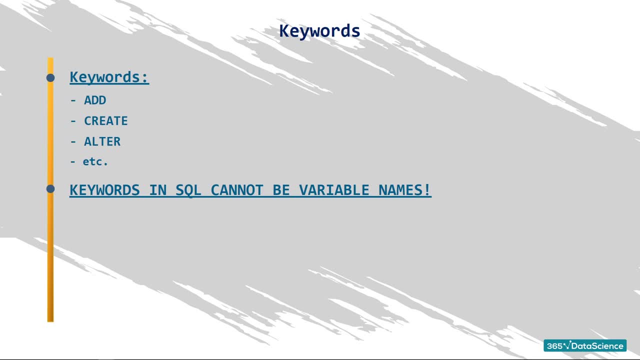 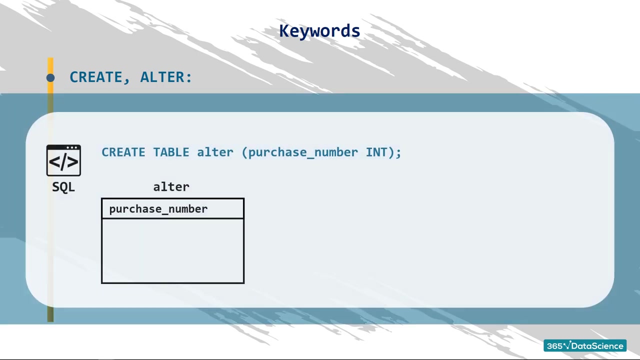 To avoid any confusion, for the software, objects or databases cannot have names that coincide with SQL keywords. To exemplify, think of all one-word statements like create and alter. They are keywords, So you can't call your table alter, since 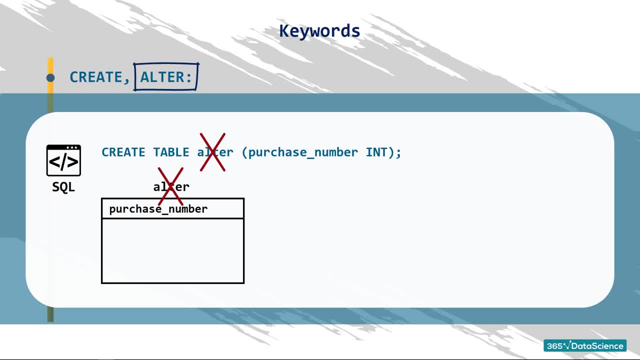 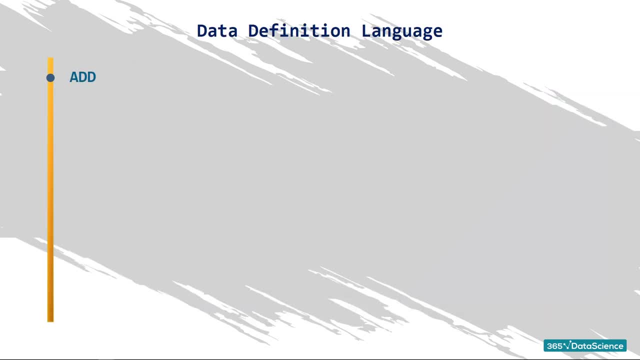 this is a name that can trigger a certain process, the modification of the content of a designated table. So back to our example. Add is the keyword that will add a column called date of purchase in the sales table. It is one of the keywords. 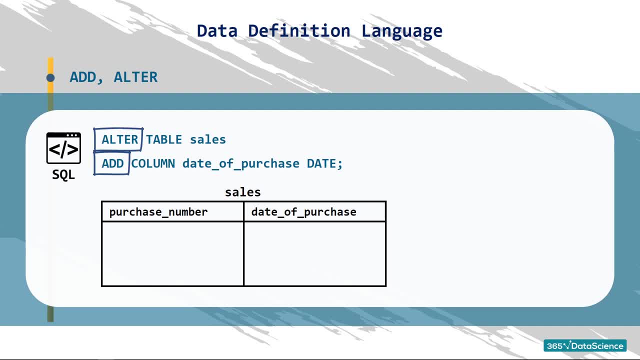 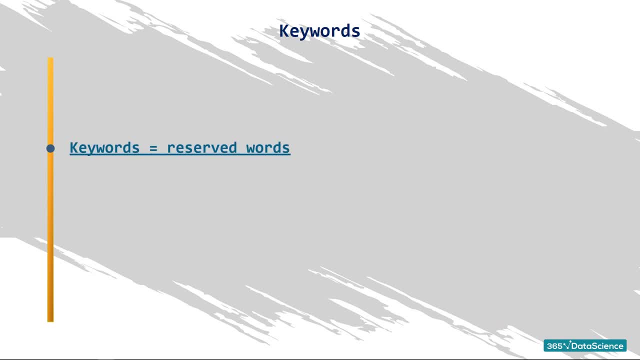 frequently used with the alter statement. Finally, don't get confused if you hear the term reserved words. It is a synonym for keywords, which indicates precisely what we explained. These words cannot be used when naming objects. Okay, so that's about it for keywords, Now that we know more about DDL and some of 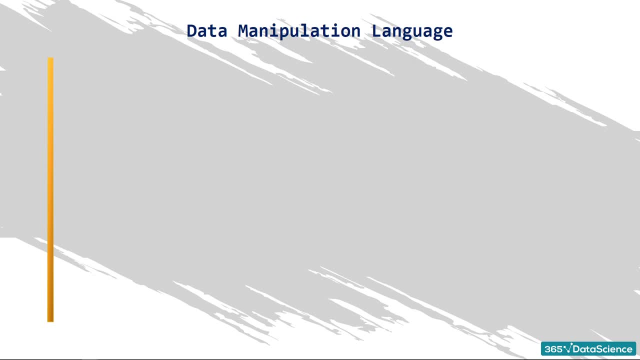 its arguments. let's take a look at some of the other keywords that can be used to manipulate data. To solve these arguments, we are ready to focus on DML, the data manipulation language. In particular, we will learn about some statements that allow us to manipulate the data in the 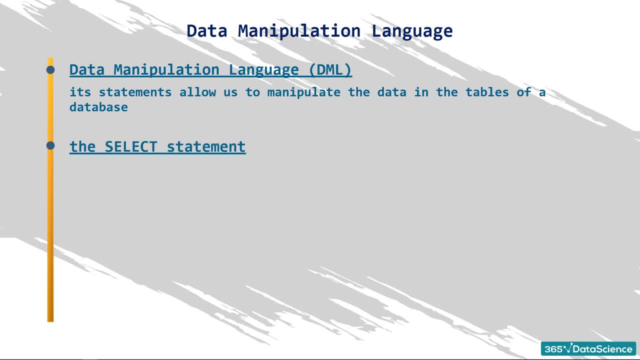 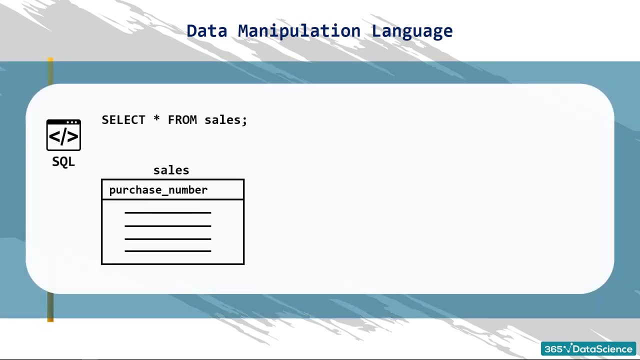 tables of a database. We will start with SELECT, a statement used to retrieve data from database objects like tables. The star after the SELECT statement in the following line will deliver the entire content of the sales table, meaning all records and fields contained in the tables. 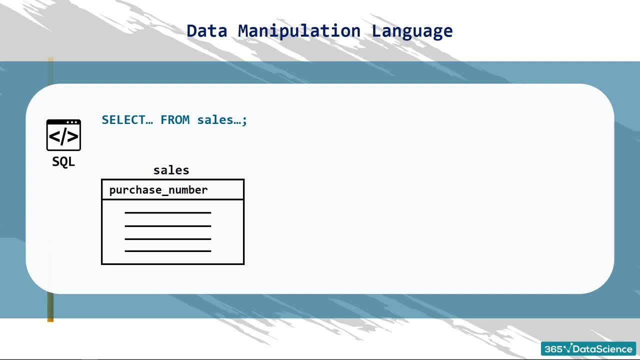 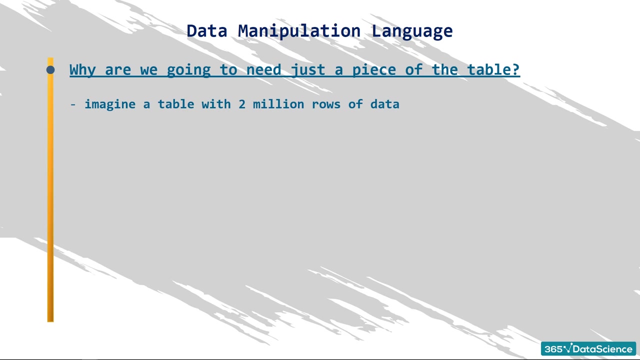 You can use the same structure to extract specific records from the table. But at this point one could rightly ask what for? We can see the entire table here. why are we going to need just a piece of it? Well, imagine a table with two million rows of data. You can only see a small part of it on the screen right. 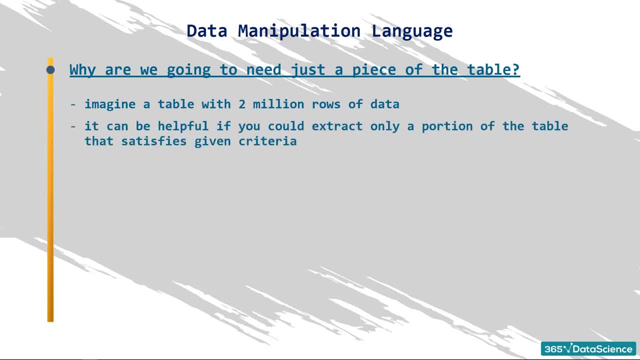 This is why it can be helpful if you could extract only a portion of the table that says the sales table. This is crucial and is one of the most powerful tools available in SQL. You should know how to use SELECT perfectly well so you designate the precise area of the table you would like to extract information from with ease. 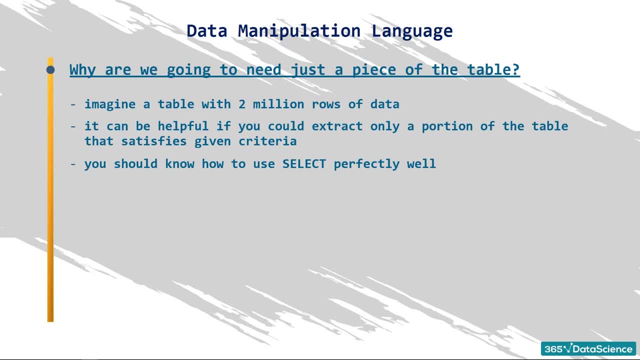 In this course. many lessons and exercises include this statement, so by the end you will feel confident when using it and selecting a certain part of a database. Insert the SELECT statement. Insert is used to insert data into tables. It enables you to add more records or rows while you are working with the table. 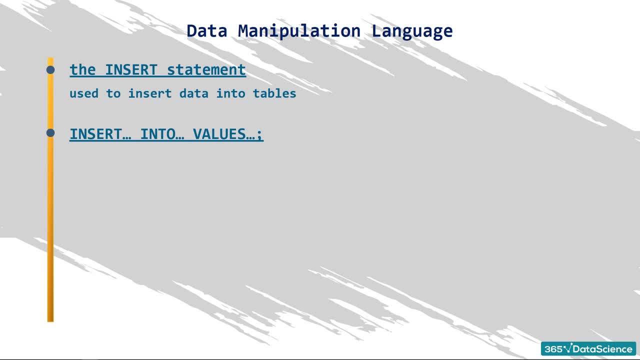 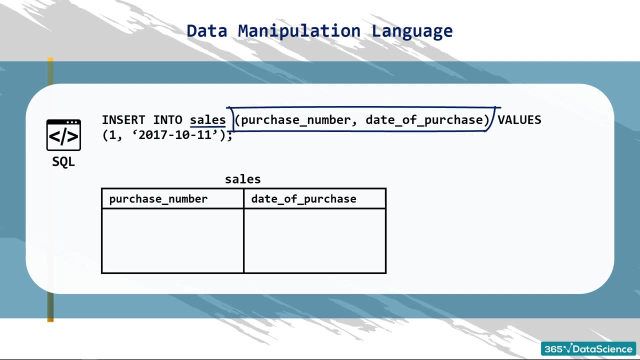 This clause goes hand-in-hand with the keywords INTO and VALUES In the parentheses after the table name. you will have to specify the columns you are adding information to, unless you want to insert data in all columns. For the moment, our sales table contains all the data. 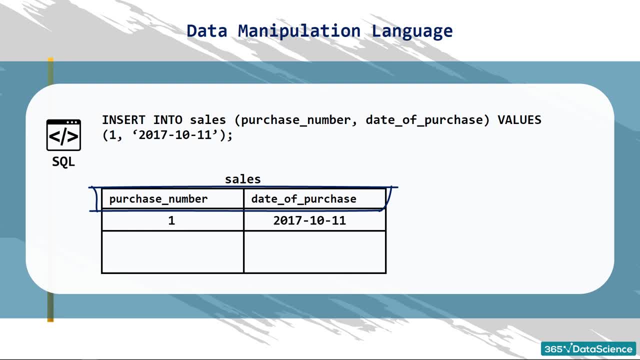 The sales table contains only two fields, So if we want to add purchase number and date values, we could omit the part with column names in parentheses and our statement would look like this: The two versions are identical Syntactically. such statement makes sense because it allows you to insert values right into a table. 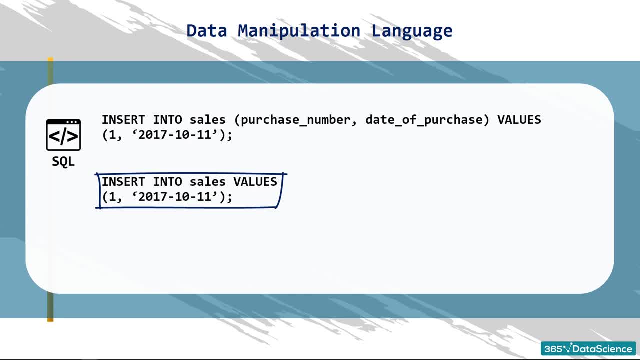 This line of code allows you to register the first record of the dataset. It will appear as the first row of the sales table. This code will add another record, purchase number 2, and the date 27th of October 2017.. 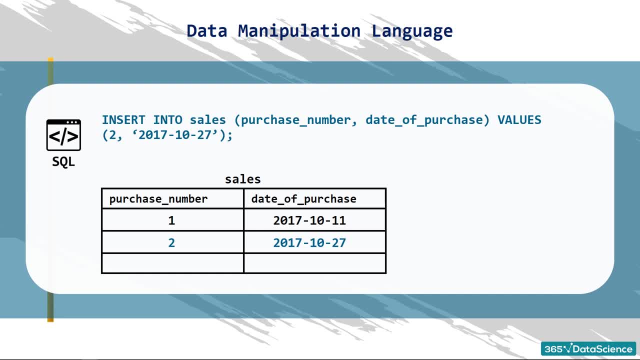 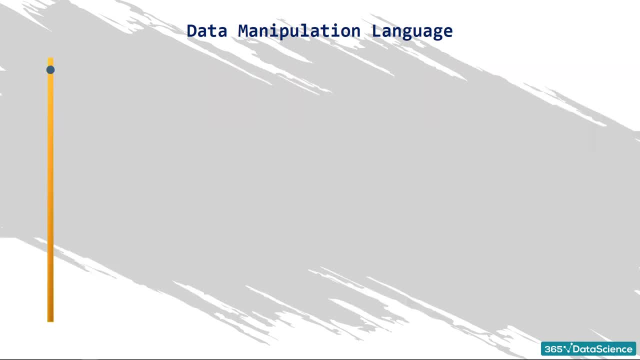 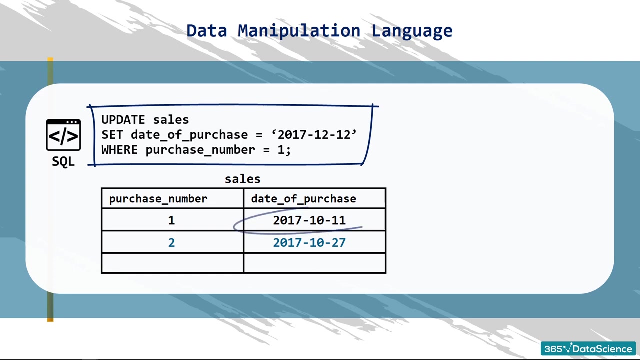 Amazing. So far we saw how to select and insert information in SQL. Remember, you can also update information. Update allows you to renew existing data of your tables. Its syntax is slightly different and is best understood with an example. This piece of code will allow us to substitute the previously inserted date of purchase number 1, 11th of October 2017, with the one specified here, 12th of December 2017.. 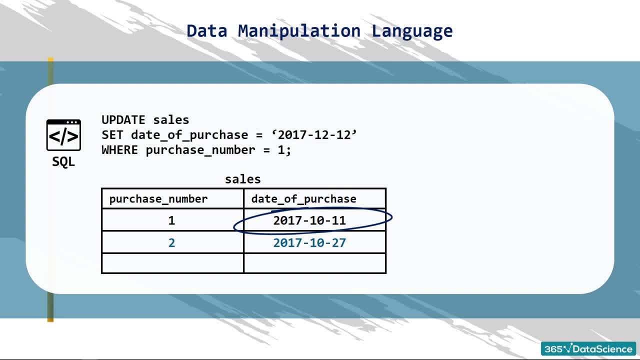 And how do we get to this date, 11th of October? The update is based on the number of the purchase: purchase number 1.. This way, the entire row is updated and the date will be 12th of December 2017.. 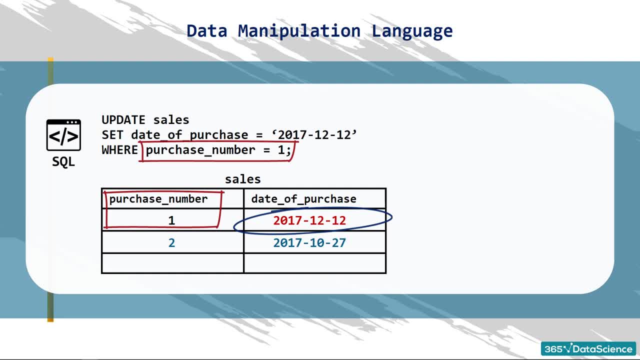 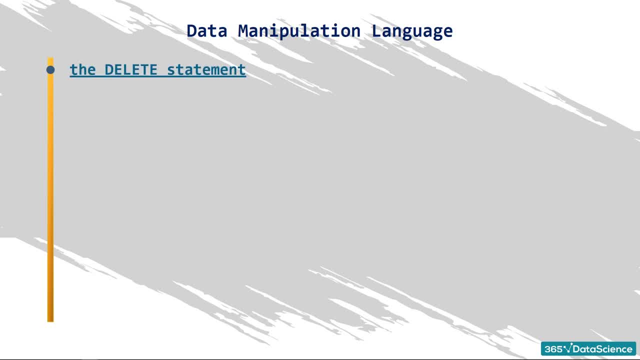 There is one additional DML clause I would like to show you in this lesson. It is DELETE. It functions similarly to the TRUNCATE statement from the data definition language, with one substantial difference: TRUNCATE allows us to remove all the records contained in a table. 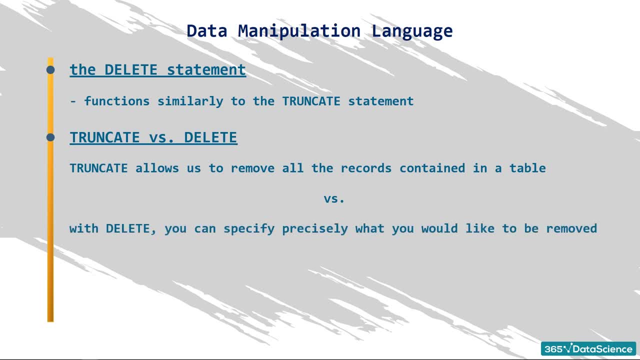 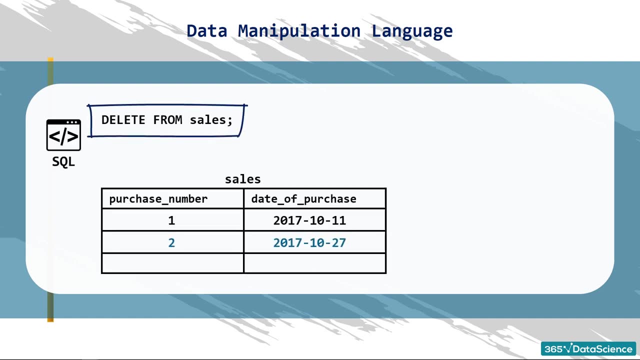 With DELETE, you can specify precisely what you would like to be removed, For instance, the following is the case, For instance, the following phrase: We'll remove all the records from the CELLS table, just as if we had written TRUNCATE TABLE: CELLS. 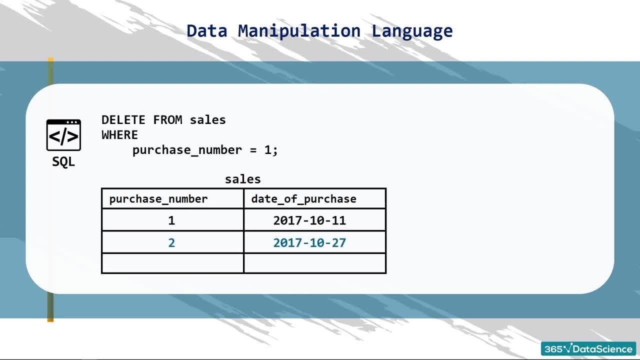 If we take advantage of the optional WHERE clause, instead the following statement: we'll delete the record with a purchase number of 1, and the other one we have in our miniature table will be left intact. Our table will remain only with the second record. 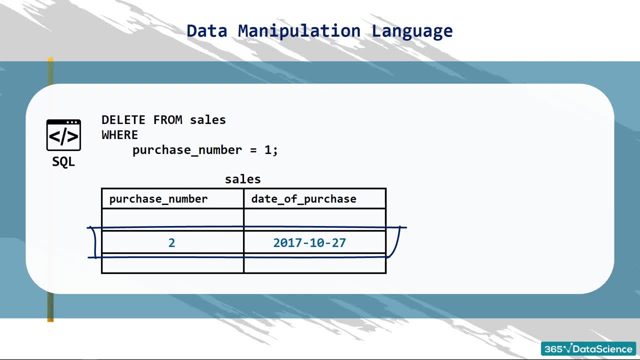 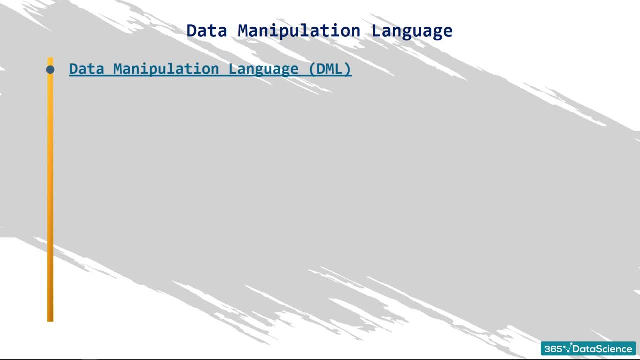 the one with purchase number 2 and date of purchase: 27th of October. To summarize the data manipulation, language syntax is composed mainly of the following four elements containing statements and keywords: SELECT FROM, INSERT INTO VALUES, UPDATE, SET WHERE and DELETE FROM and, optionally, WHERE. 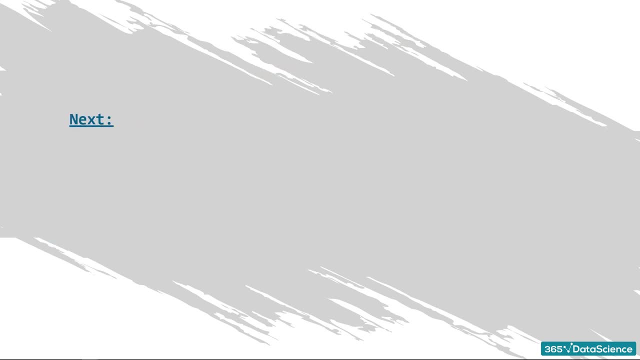 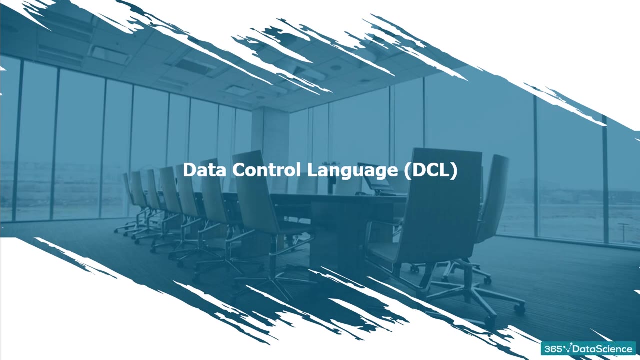 In our next video we'll learn what part of SQL syntax is referred to as data control language. The data definition and the data manipulation languages are probably the ones you will use more often. The following two lectures are rather informative. Some terms we will use will not be used later in the course. 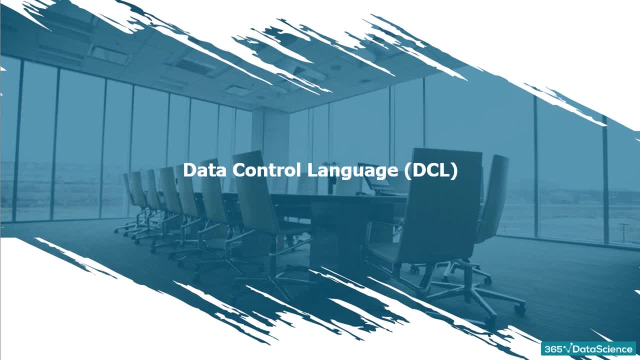 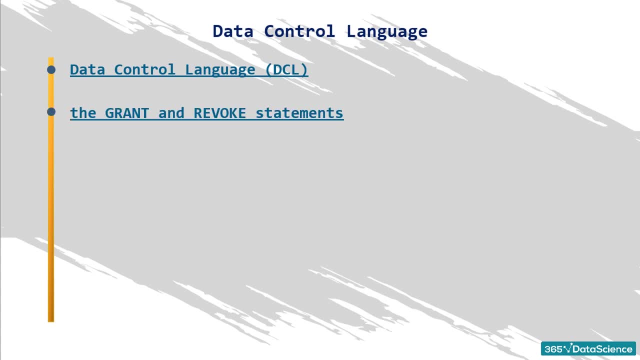 However, please pay attention, as they will widen your view about the activity domain of SQL. The data control language is a syntax containing only two statements: GRANT and REVOKE. As you probably guessed, these statements allow us to manage the rights used in the data control language. 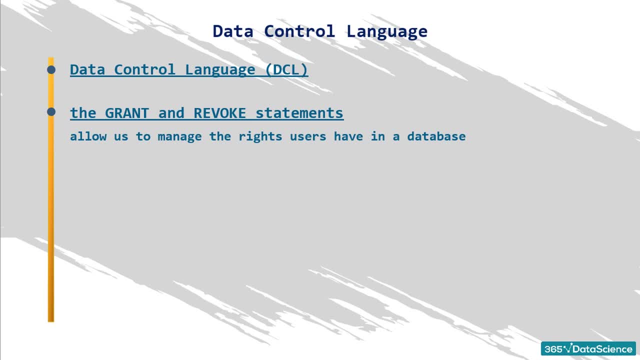 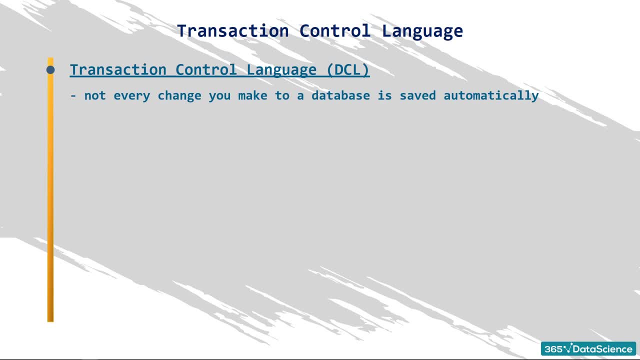 As you probably guessed, these statements allow us to manage the rights used in the data control language. As you probably guessed, these statements allow us to manage the rights used in the data control language. You have to say you wish that to happen. The statement to use in such cases is commit. 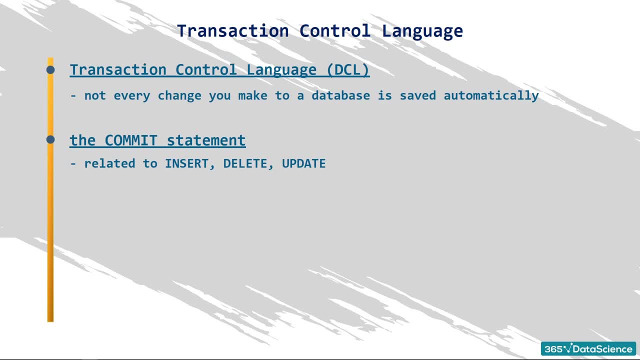 It works only for changes made with the help of the insert, delete or update clauses. Commit will save the changes you've made permanently on the database and will let other users have access to the modified version of the database. For instance, imagine you have updated a record in the customers table. 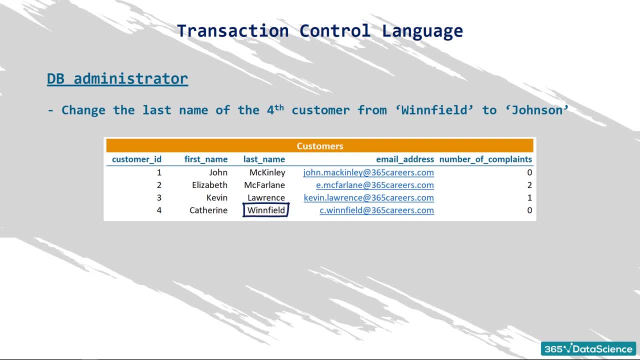 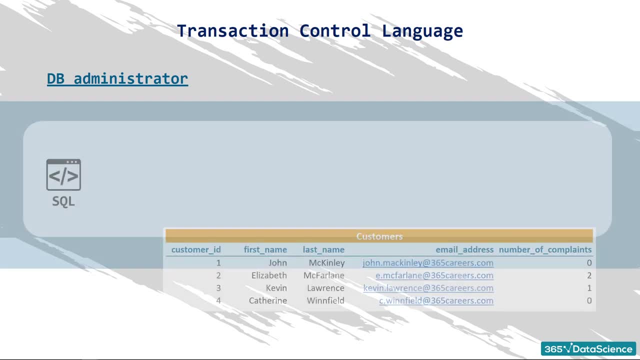 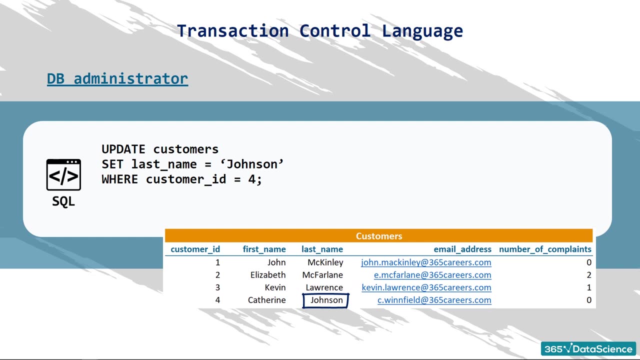 Say you wish to change the last name of the fourth customer from Winfield to Johnson. If you are an administrator you can do that with the help of the update clause And you will see Johnson appear in the place of Winfield. The update statement we saw earlier would allow you to change the last name of the fourth customer. 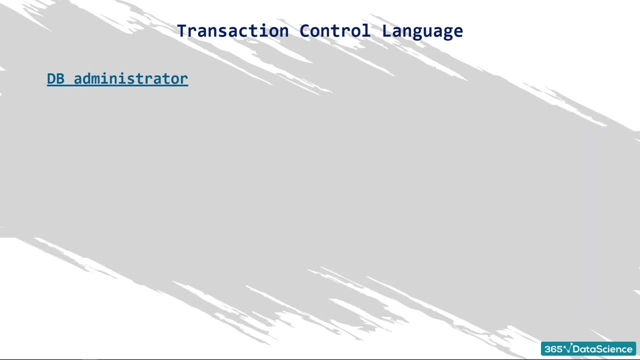 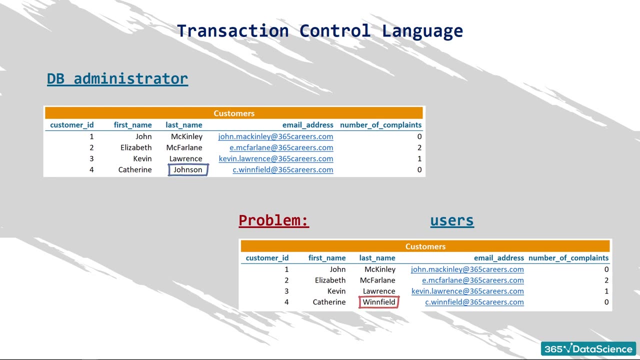 However, your work isn't done just yet. The rest of the users working with the database system cannot see you have made any changes. To complete the entire process, you must add a commit statement at the end of the update block. To complete the entire process, you must add a commit statement at the end of the update block. 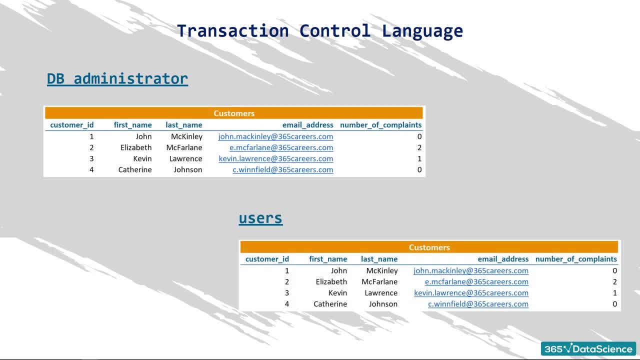 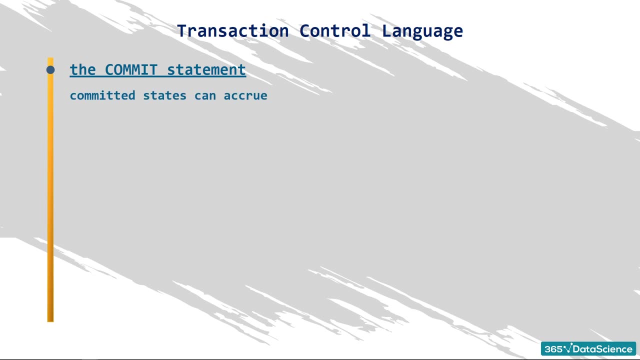 Only then will the updated information be available to all users. They will see Katherine Johnson, not Katherine Winfield, as customer number 4 in the customers table. Committed states can accrue. If you are a database administrator, you might need to use commit 20 times per day. 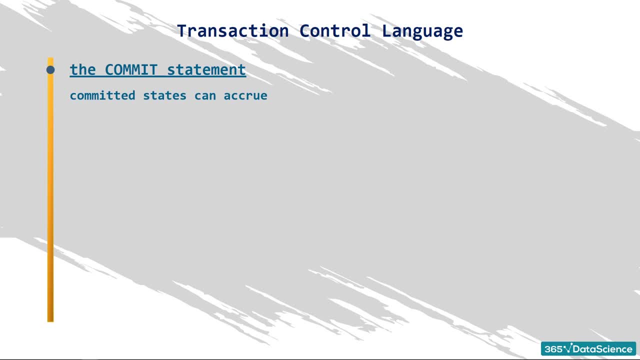 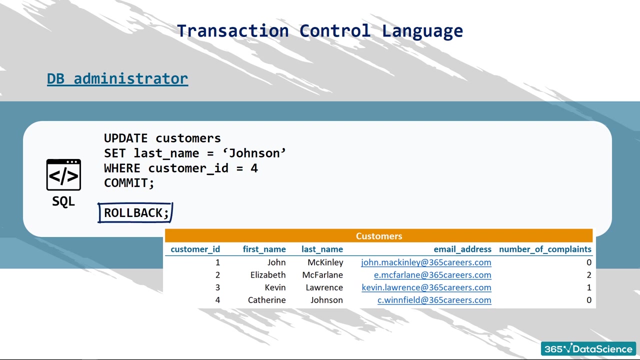 The transaction control language clause that will let you make a step back and restore the database to the last committed state is rollback. This allows you to undo any changes you have made but don't want to be saved permanently. To apply this command type: rollback. 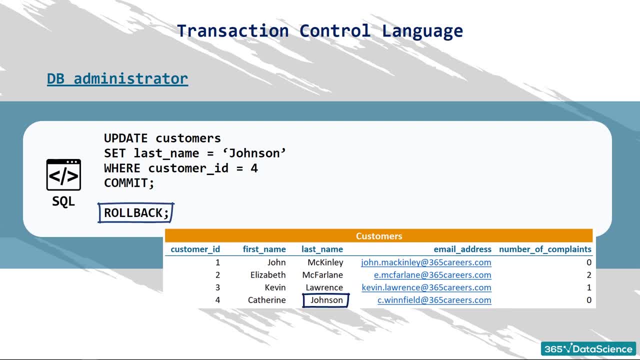 Be careful when using this statement, because it will revert to the last committed state and all the changes made in the meantime will be removed. There can be multiple statements executed and they will all be undone. To recap: commit saves the transaction in the database.